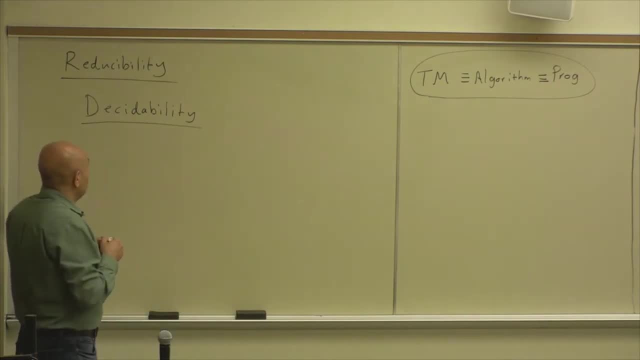 So this is the kind of description that we are using in this part of the course. Now again to review. you know we looked at regular languages. You know we're looking for algorithms related to regular languages- context-free languages. 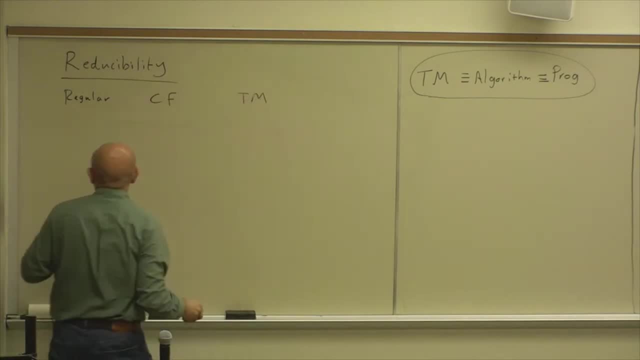 And Turing machines And we looked into the acceptance problem for DFAs and the empty problem for DFAs and the equivalence problem for DFAs And all of these are decidable. We showed that all of these are decidable. They have algorithms for solving them. 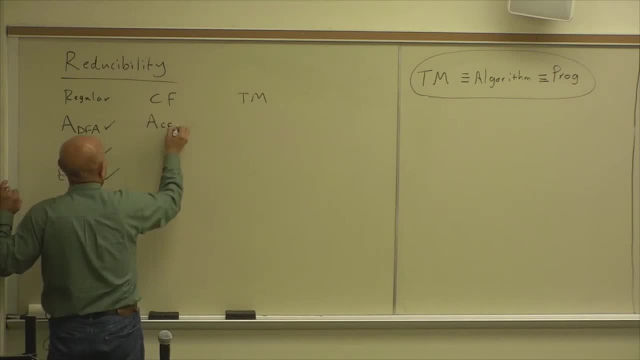 We looked into context-free grammars. The acceptance of context-free grammars is decidable. The emptiness of context-free grammar determines the value of the grammar. So we looked into context-free grammars. We looked into context-free grammar. We looked into context-free grammar determining. 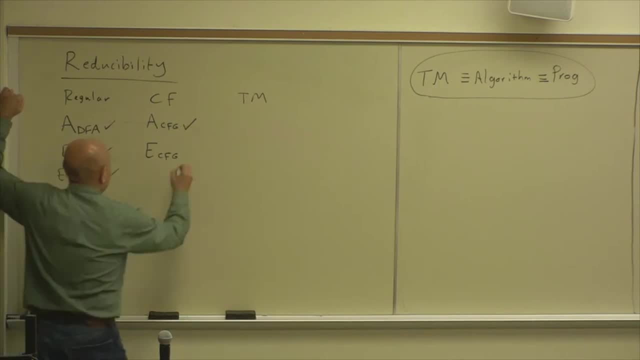 if a language is empty. Was that decidable or not? Yeah, It was decidable. And what about the equivalence of context-free grammar- Not decidable? No, It's not decidable. Now, last time we looked into the first problem related. 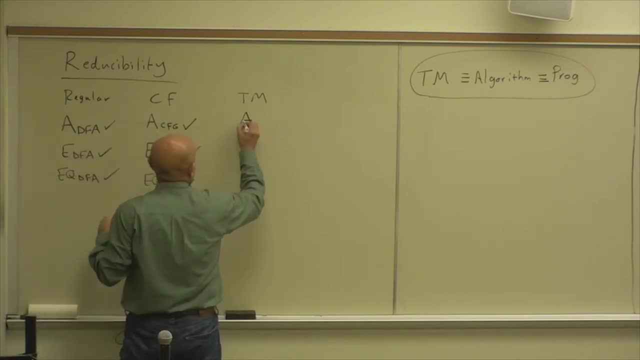 to Turing machines or algorithms or programs, The acceptance of Turing machines. And was that decidable or not? No, it was not decidable, So we did not give the actual proof, but I tried to explain intuitively why acceptance is not decidable. 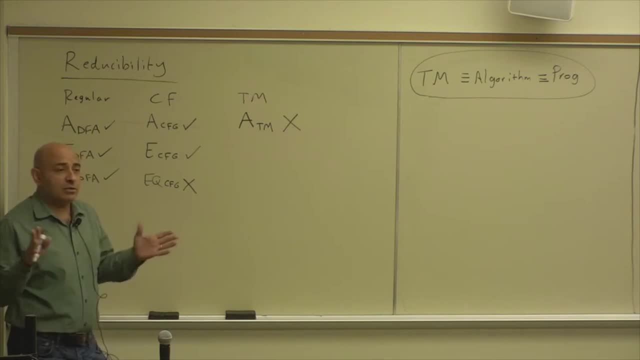 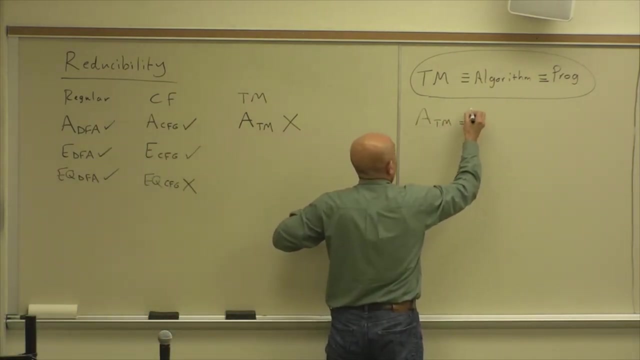 and what. who can summarize that intuition behind this? What's the intuition behind you know, ATM is not decidable, accepting So ATM is. you are given a Turing machine and a string and the objective is to determine. you know. 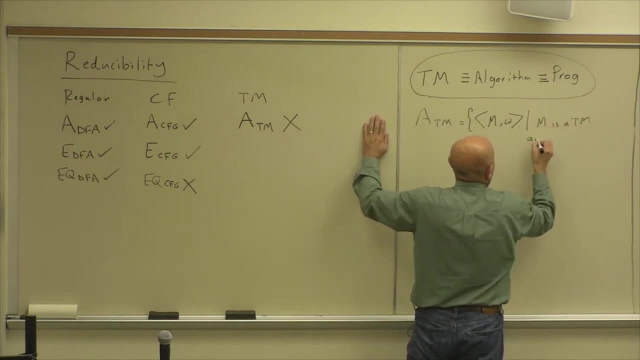 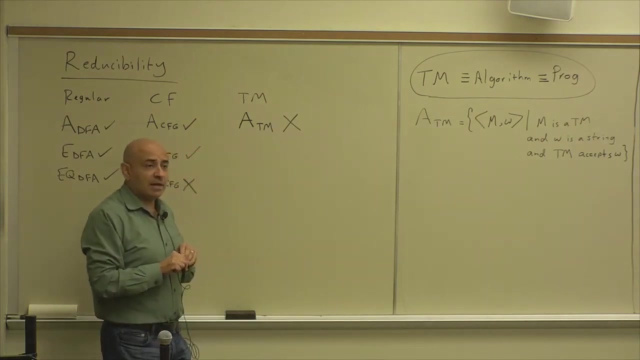 M is a Turing machine and W is a string and TM accepts W, Determining if TM accepts or rejects W. What was the intuition? So what kind of program is this? So we're writing an analysis program that takes another program and it takes an input and the objective. 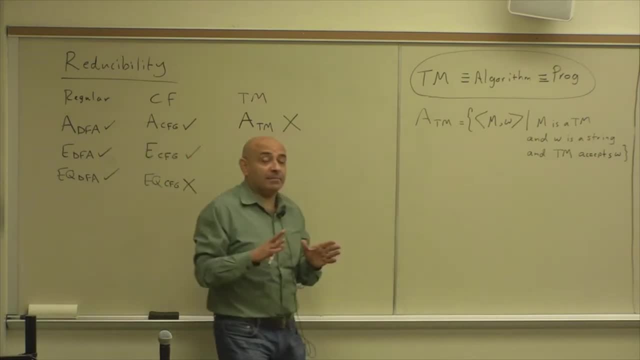 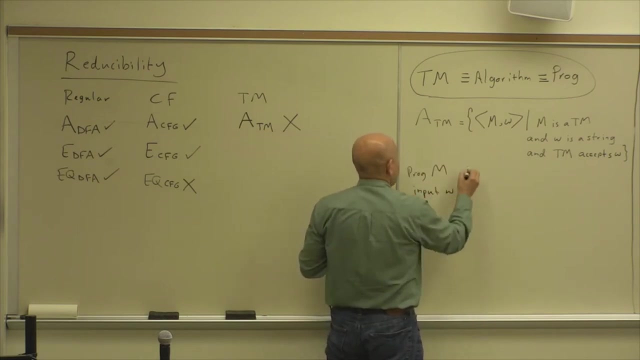 of this analysis program is to tell you within finite time if program M is going to output a yes for string or for input W. So the objective is writing an analysis program that takes program M and input W and determines in finite time if, with input W, output is yes. 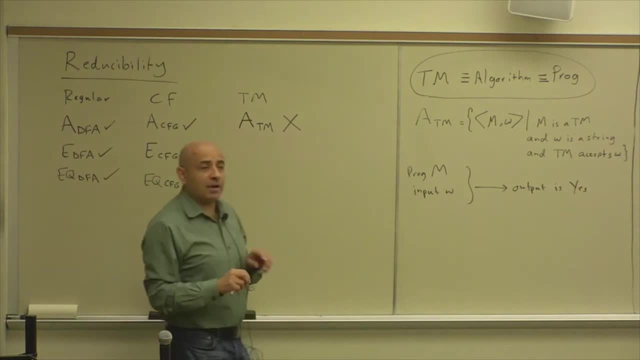 So program M is a program, that whose output is either yes or no, And the objective of the analysis program is to determine whether program X will output yes if we input W in it. And, as we'll show today, this is, you know, the challenge. 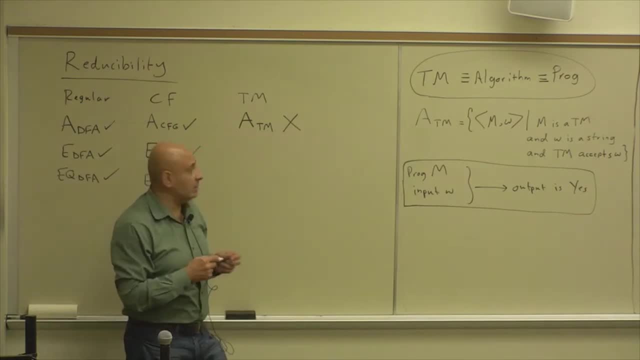 in doing this is determining if M is going to hold. 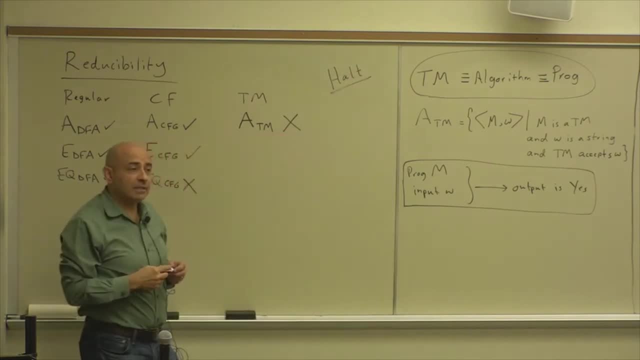 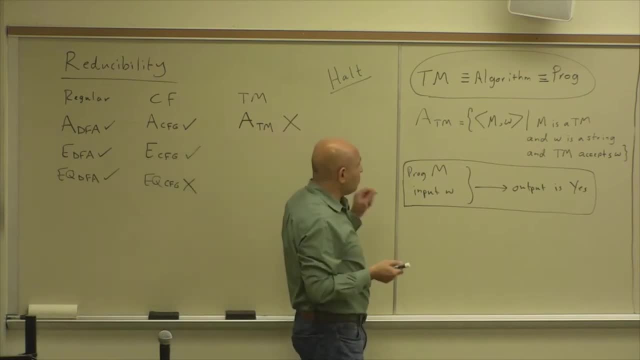 the intuition is that program M is a general program. Basically, it's written in the same general or in a general purpose language. that's as powerful as the program, as the language in which we wrote the analysis program. 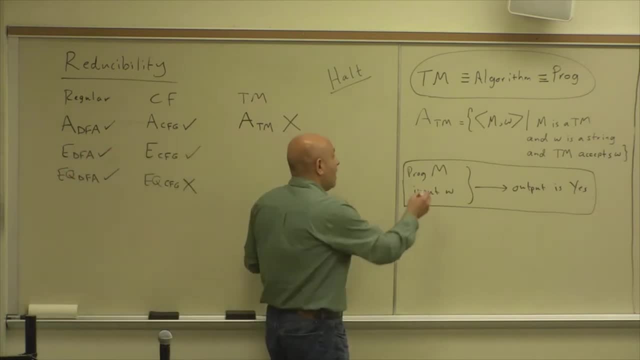 So the analysis program that we're trying to write and the program M that we're trying to analyze. both are written in general purpose programming languages. Of course they don't have to be written in the same language, But they both have to be written. 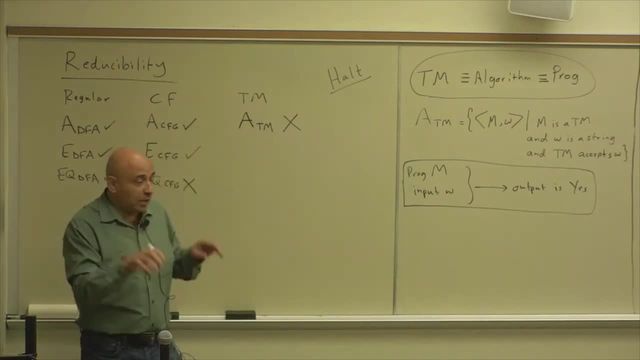 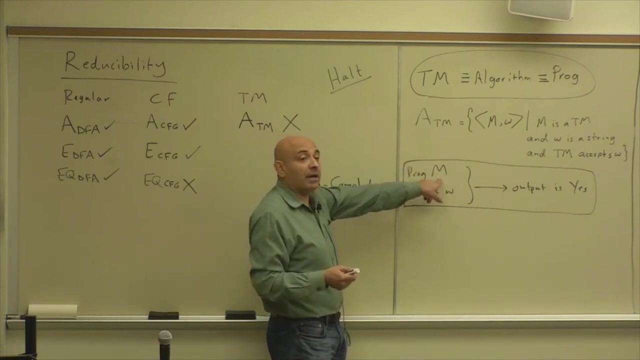 in general purpose programming languages or Turing complete. Turing complete programming languages, a language that has all the features that can be implemented using a Turing machine. okay, The problem lies in the generality of the program that we are trying to analyze. So that program that we're trying 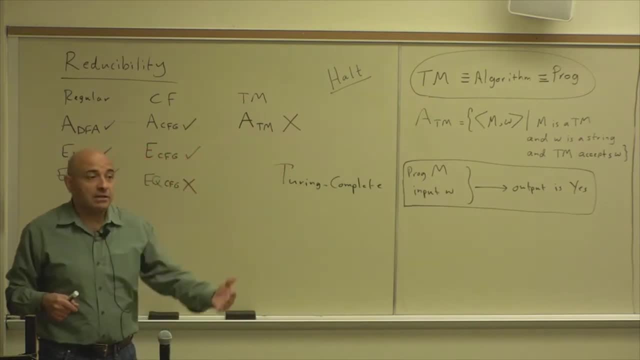 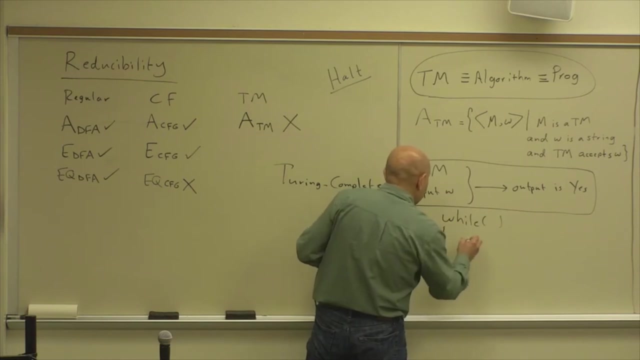 to analyze, may have all kinds of function calls and recursions and loops, and the condition for terminating loops or the base conditions for recursion may be very complex. So you just have a loop and then in that loop if complex expression, break This complex expression if the language is general enough. 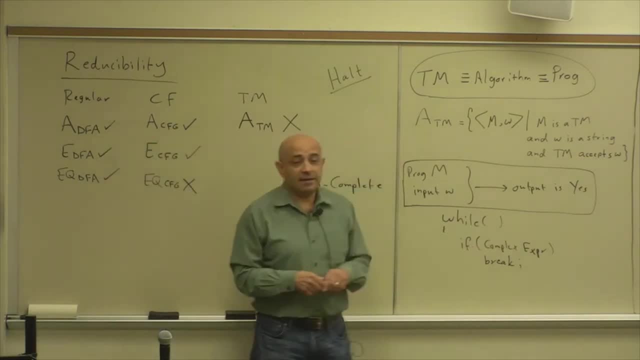 can be very, very complex, right, It can have many, many function calls or many, many levels of function calls in it. All right, so analyzing it in general is not possible. Analyzing a general program is not possible. Okay, so that summarizes the intuition. 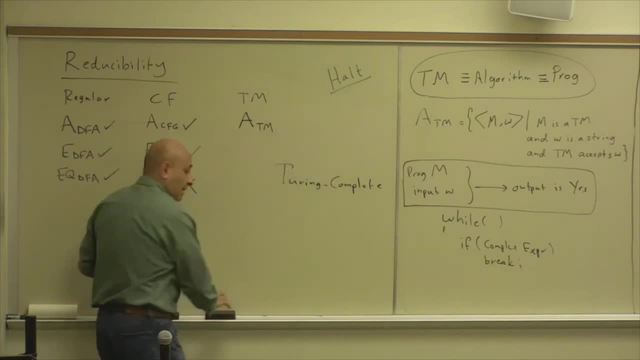 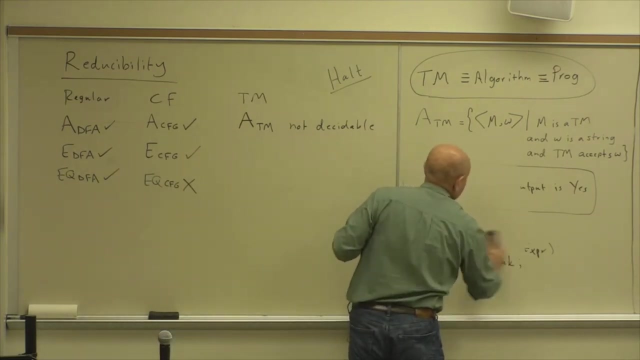 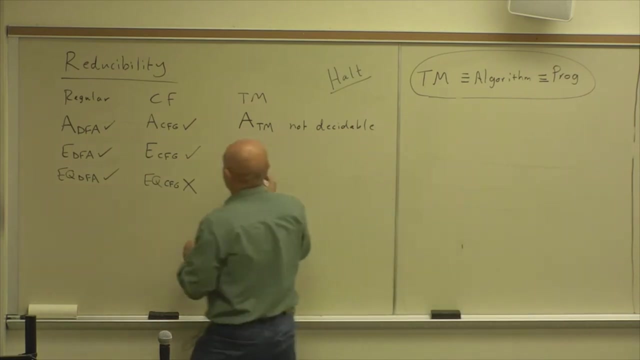 behind ATM is not decidable. Okay, Now, today we will Look into, you know, the other two problems, which are ETM and equivalence of TM, to see whether it's decidable or not. But before that, we will look into this problem. 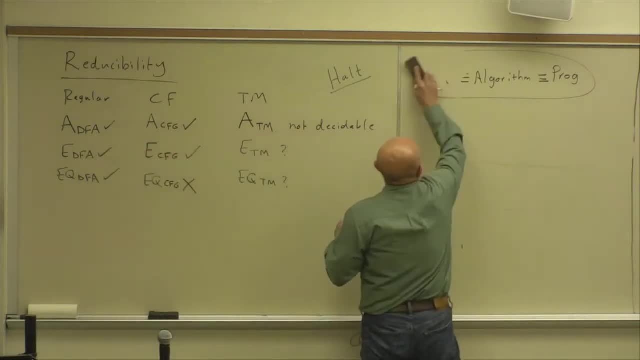 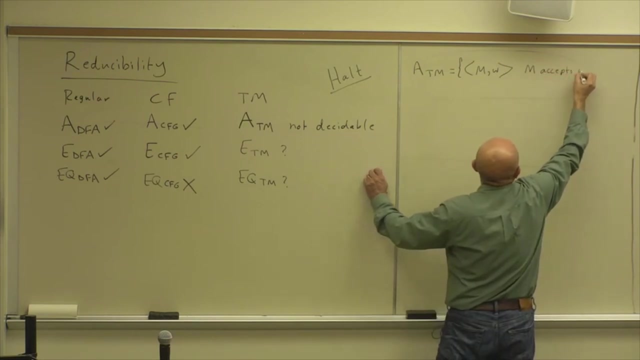 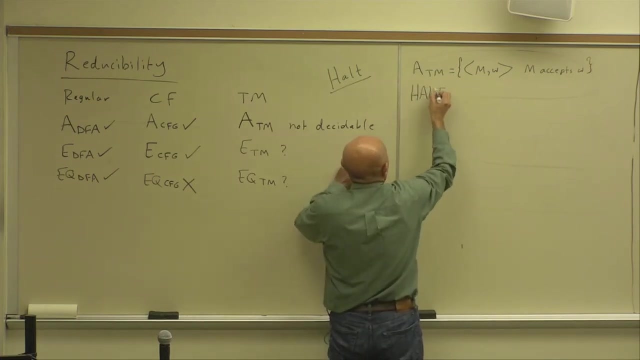 which is the halting problem. So Well, first, ATM is Given M and W. M accepts W, where M is a Turing machine, W is a string and halt TM is given a program M and string W- M halts. 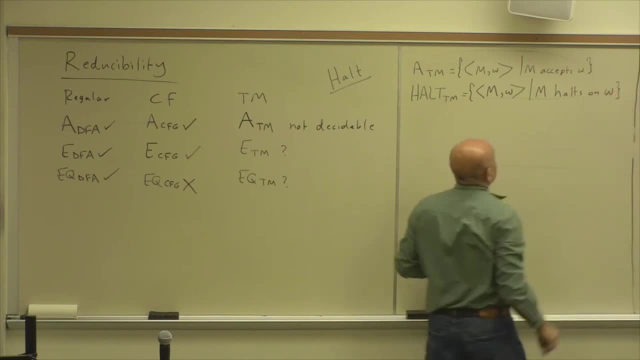 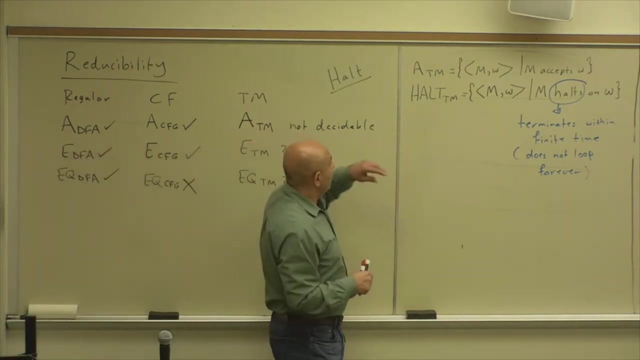 Now what does halt mean? It means it terminates within finite time. So halts means terminates within finite time. Or in other words, does not loop, Does not loop forever. Okay, Now we will show how, if we assume that ATM. 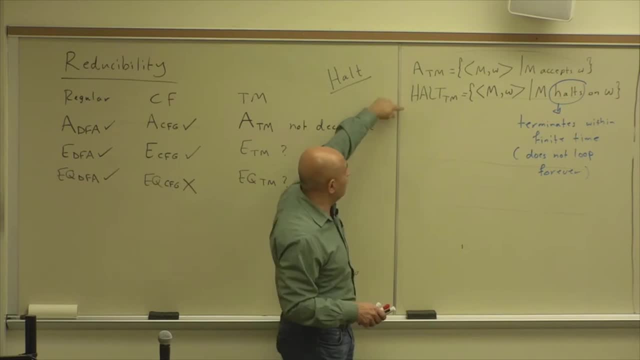 the acceptance is known to be undecidable. how we can prove that the halting problem is undecidable? And this can be proved using what we call reductions. Now, what's a reduction? A reduction is a way of Converting one problem to another problem. 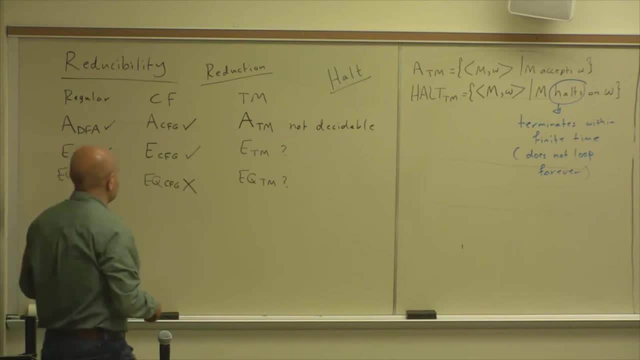 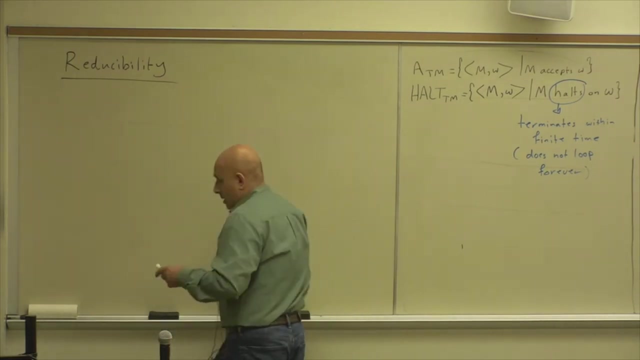 And in order to explain the concept of reductions, I'm going to use problems, different kinds of problems that you are familiar with. I'm going to use the cubic equation problem. So Let's assume that we have a program or an algorithm. 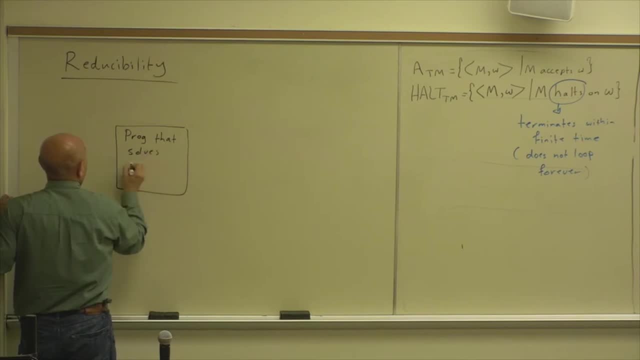 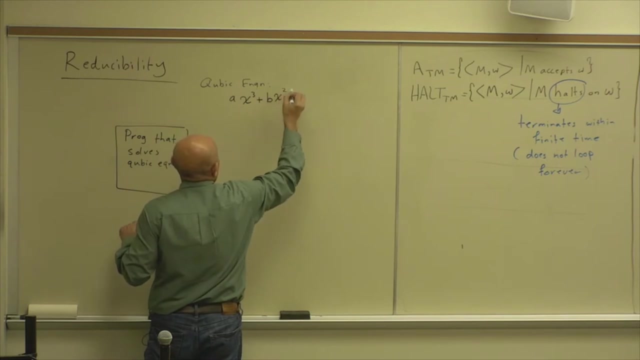 Let's assume that we have an algorithm that solves cubic equations. So a cubic equation is of the form: AX cubed plus BX cubed squared plus CX plus D equals 0. So this program, you give it A, B, the coefficients of the equation, A, B, C and D. 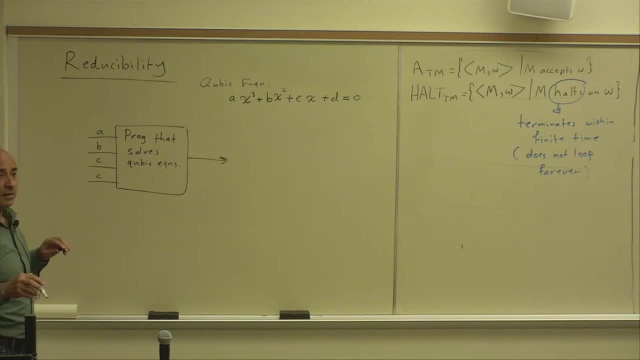 And what does it give you? The roots, The values of X, Or roots solutions, Or the solutions- The values of X, Or roots solutions, The values of X, which satisfy this equation. So this is a program that solves this equation. 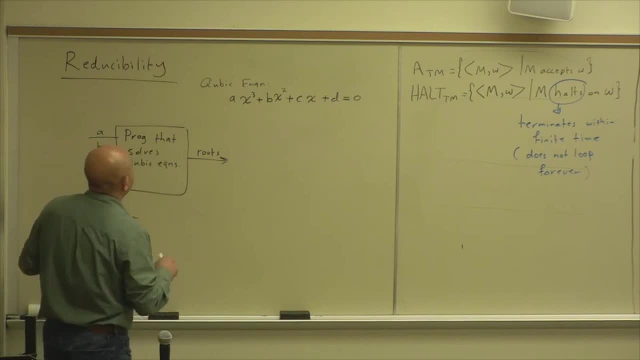 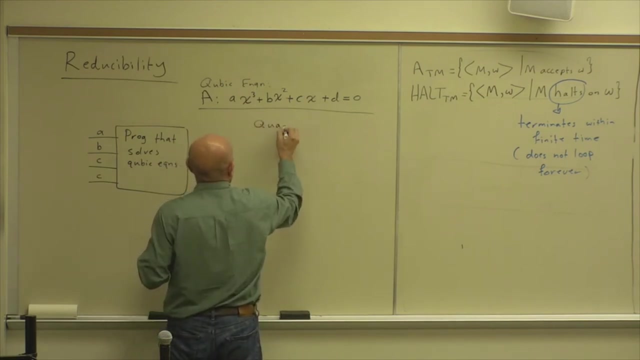 Now let's call this problem problem B, Or problem A: Y. Now what about the quadratic equation? This is equation Problem. Let's call it problem B, Where we have EX squared plus EF, plus FX, plus G, EFG equals 0.. 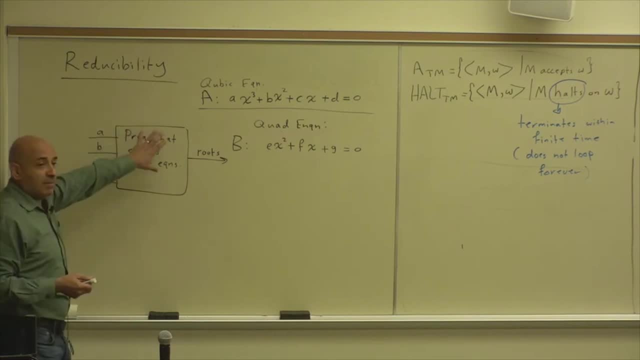 Now if I give you this program that solves cubic equations, So let's call it problem B, Where we have EX squared plus EF, plus FX, plus G, EFG equals 0.. Now what? if you solve a cubic equation, Can you use it to solve quadratic equations? 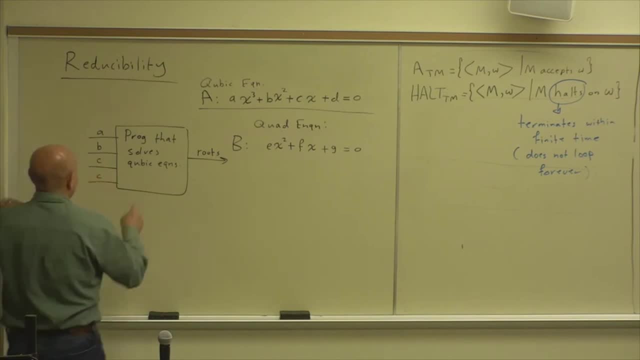 Yeah, You can easily use it Now in order to use this solver for cubic equations to solve Solver for cubic equations, to use it for solving a quadratic equation, what should you set A to A to 0.. Yeah, You set A to 0. 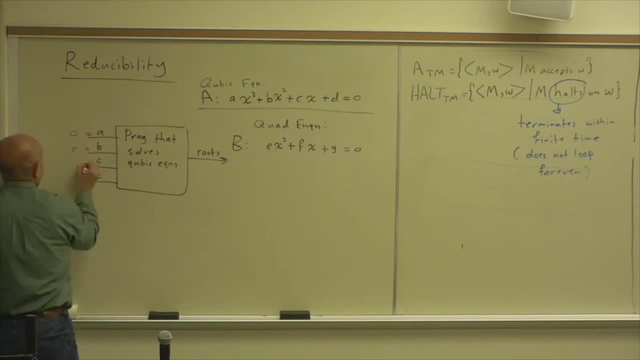 You set B to E, E, And you set C to F, and then you- and this is D, sorry- And you set D to G. So you are given this solver for cubic equations. You use it to solve quadratic equations. 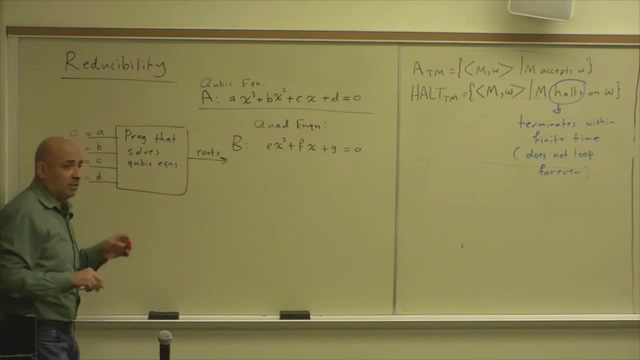 So this is a reduction, but this is a very easy reduction, because all what you needed to do is to set the values of these coefficients. So in this case, you know, we say that B is reducible to A, So we manage to reduce the problem. 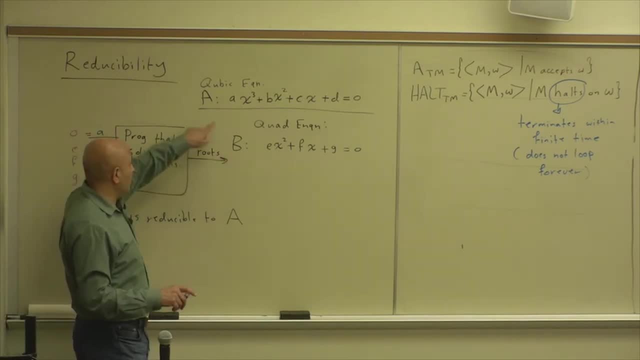 of solving B into the problem of solving A, Or given a solver for A, we manage to solve B. Now, the term, the term is a little bit complicated. The notation that we will use, B, is less than or equal M. In fact. 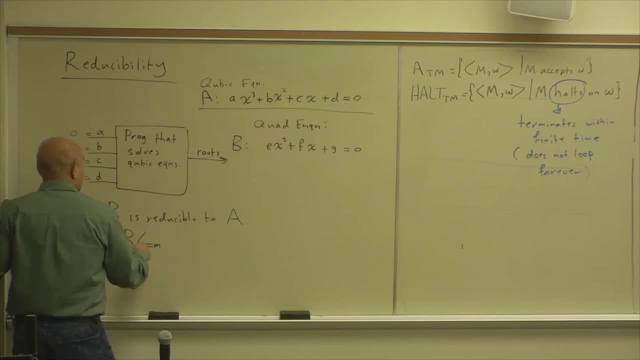 we don't read it less than or equal. We read it reducible, mapping reducible to A. So this, we read this as mapping reducible. What does mapping reducible mean? It means that there is a mapping, a function, mapping reducible. 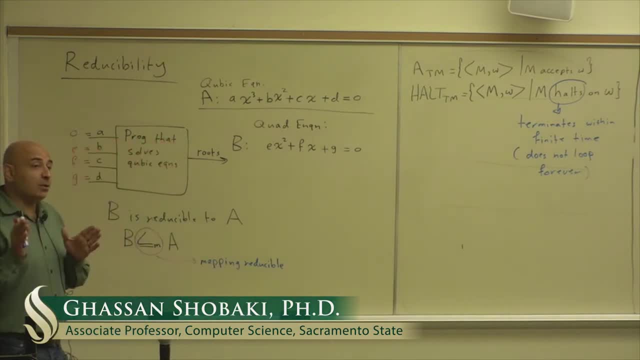 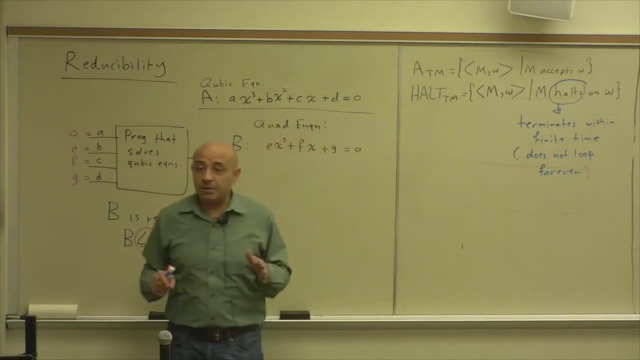 There is a function, and that function is Turing computable. We can compute it using a Turing machine or we can compute it using, you know, a general purpose, a program written in a general purpose language, running on a general purpose computer. 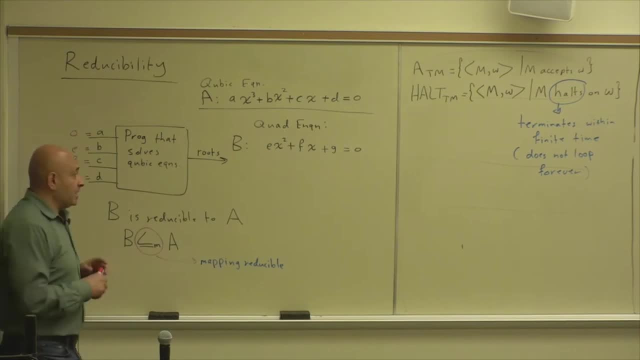 And we know that. you know what the operations, that a program written in a general purpose language running on a general purpose computer, what the operations are You know. we know that a general purpose computer can easily do all kinds of arithmetic: add, subtract, multiply, divide. 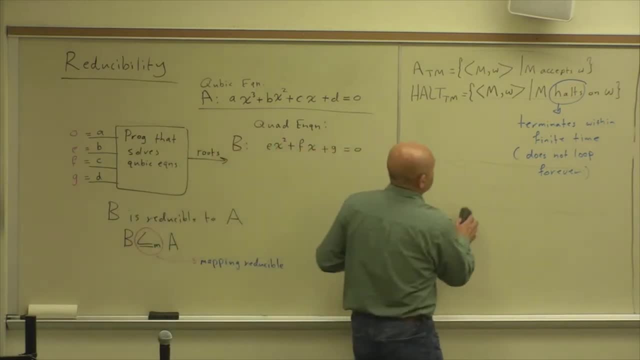 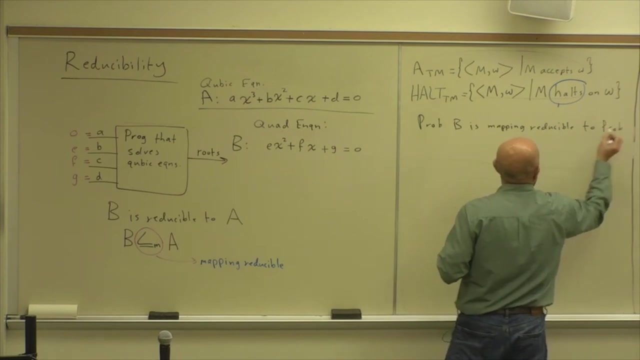 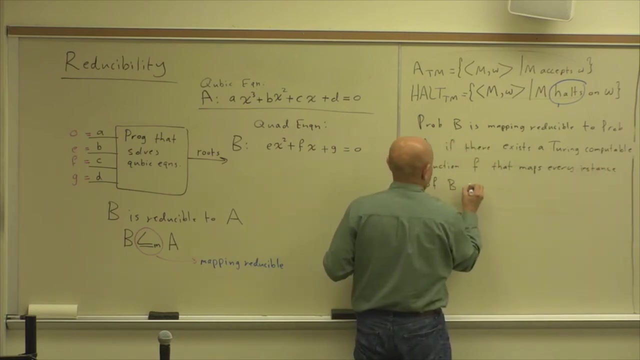 etc. So problem B. Problem B is mapping reducible to A or to problem A if there exists a computable or Turing computable. Now let's move on to function function F That maps every instance of B into an instance of A. 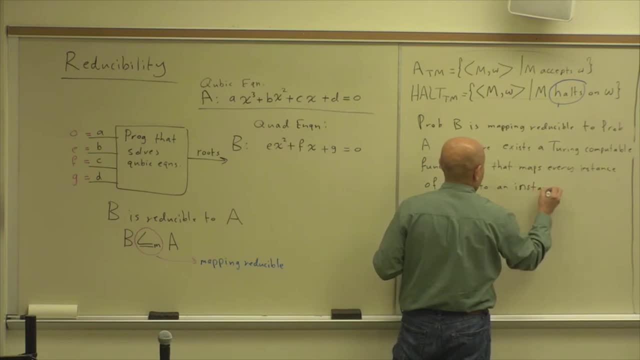 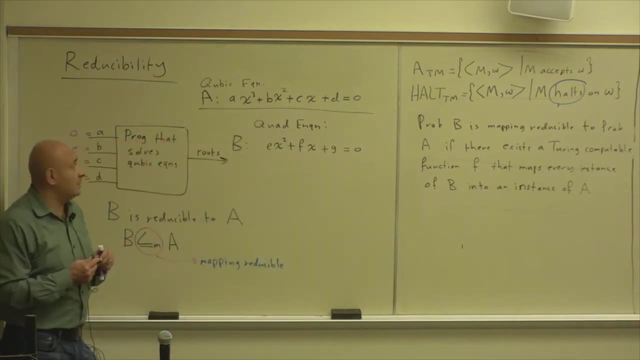 Perfect, Thank you, Let's move. All right, Perfect, Good job. OK, gehabt. OK, All right, Good job, All right. So, given an instance of B, any instance of B can be converted into an instance of A. 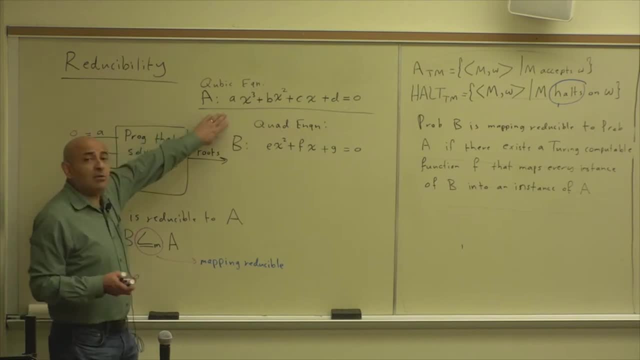 By the way, in this, for this example, can we do the mapping in the other direction? Can we map every instance of A into an instance of B? No, we cannot, because in this case B is just a special case of A, A is a more general. 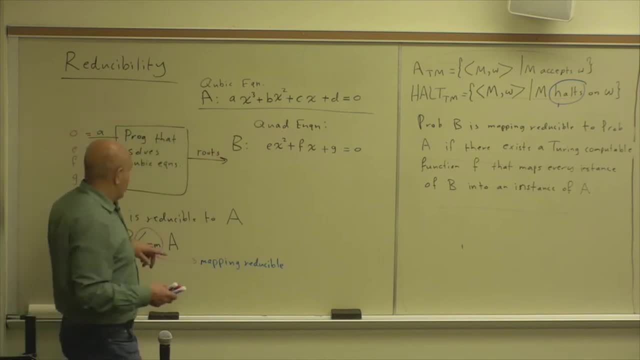 problem than B. Now, this relation, mapping, reducibility, is going to exist between two problems or two languages, not only when one of them is a special case of the other or one of them is more general than the other. In fact, they can be on the same level. 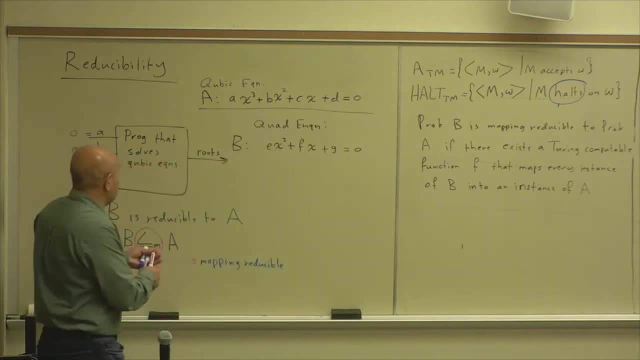 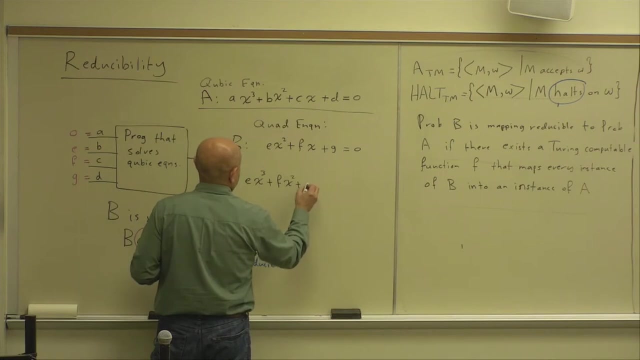 They can be different forms of the same problem. So I can give you problem C, for example. Problem C. Problem C is, you know, E X cubed plus F X squared plus G X equals H. So now, intuitively, 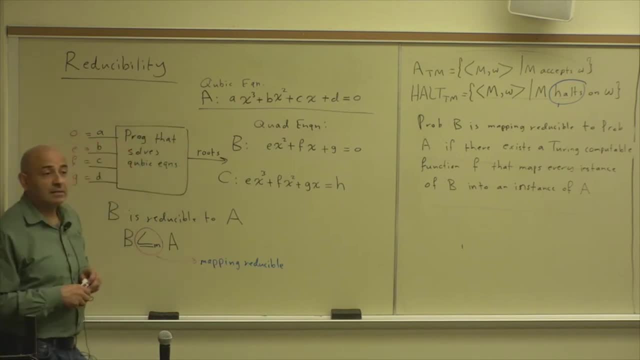 you know what's the relation between problem A and problem C. It's the same problem, right, But in two different forms. Now, if I have a solver for A, I can use it to solve C by setting A to E and B to F, C. 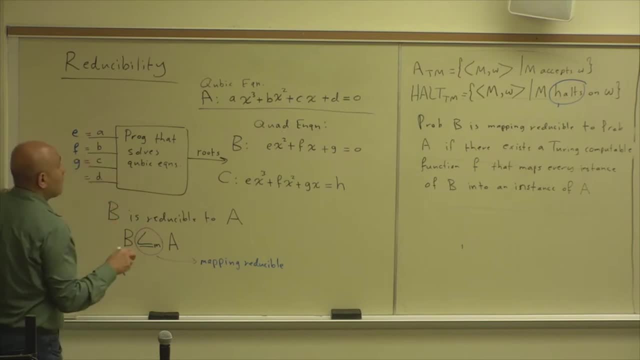 to G and D. It's going to be the same problem in two different forms. The same problem is going to be the same problem of A and B. 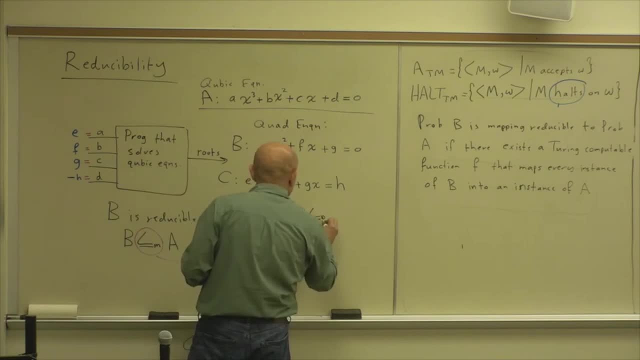 And in fact we can do the do it in the other direction as well. If we have a solver for C, we can also use it to solve A. So it you know it can. 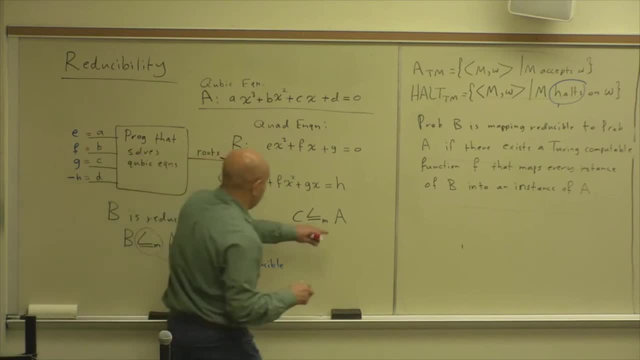 the relation can go in both directions. So C is reducible to A and A is reducible to C, because in this case A and C are two forms of the same problem, While this bidirectional relation does not exist between A and B. You know, B is reducible to A. 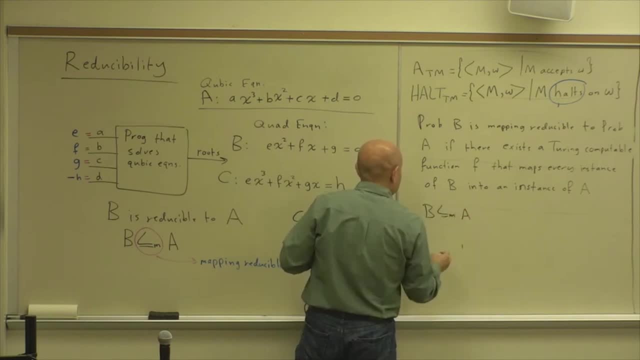 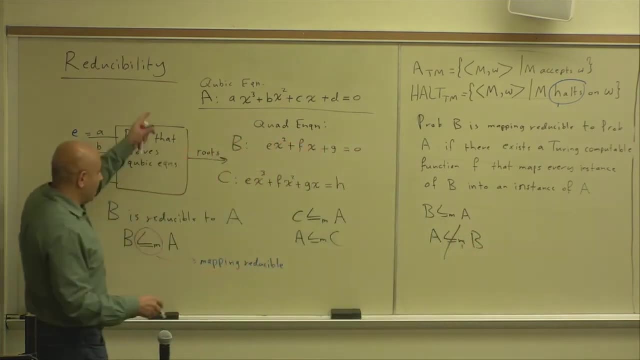 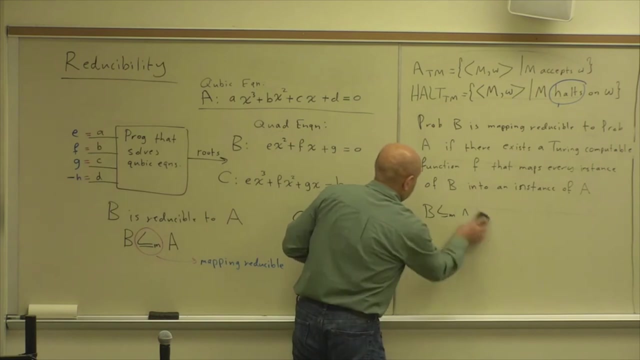 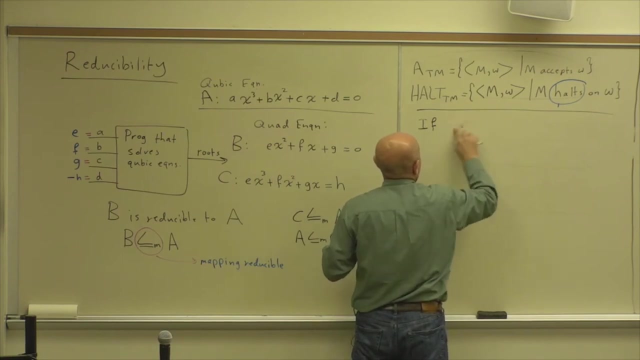 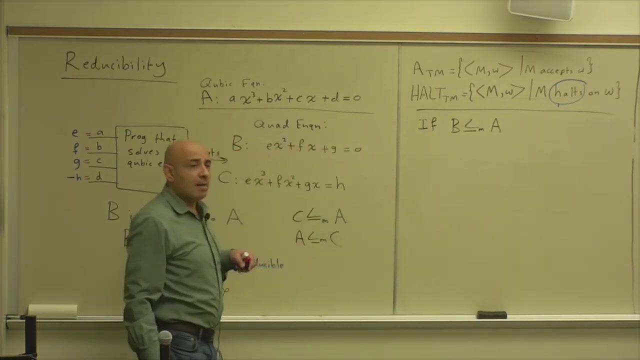 but A is not reducible to B Because A is a is a more general problem. Okay, Now how does this help us prove that a certain problem is decidable or undecidable? Now let's see If, if problem A, or let's A, is polynomial, or let's do B- B is mapping reducible to A And A is decidable. 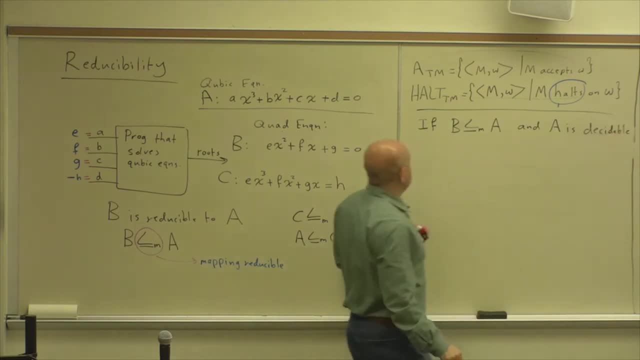 What can we say about B? B must be decidable because we can reduce any instance of B into an instance of A. So if A is decidable, it means there is an algorithm for solving A. If there is an algorithm for solving A, I can always use it to solve B, because this means that I can convert any instance. 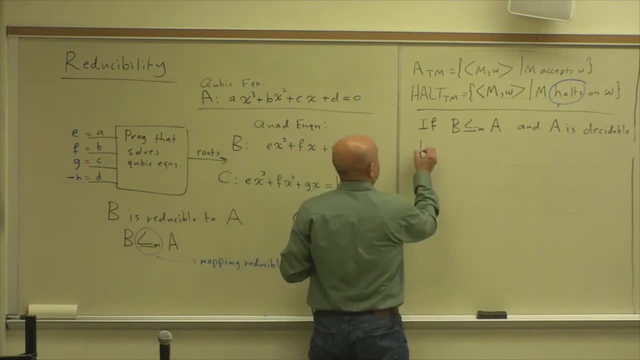 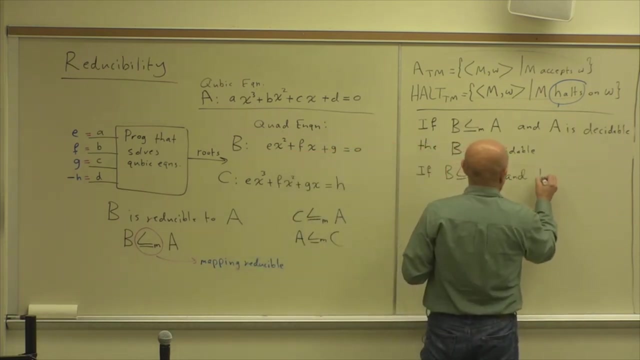 of B into an instance of A. Okay, So this implies then B is decidable. Now, if B is polynomial, is mapping reducible to A and B is not decidable. what can we say about B? Okay, Okay. 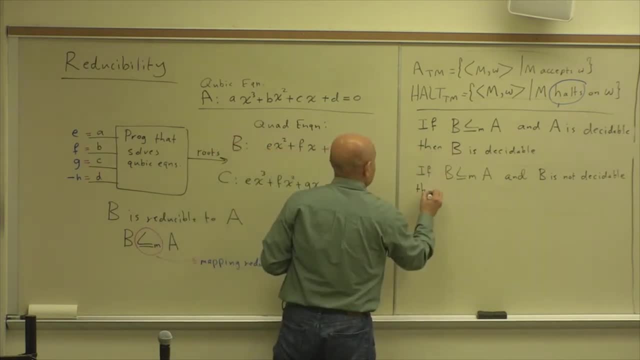 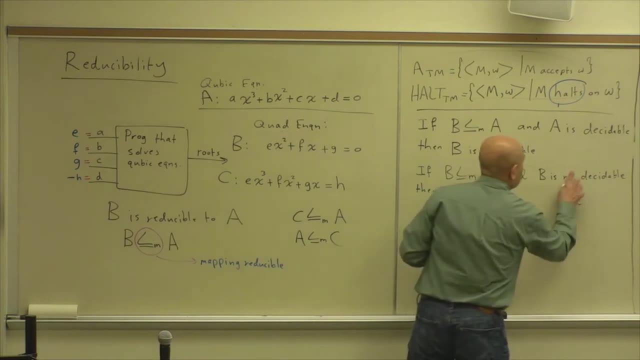 Let's start Now. if we go from A to B, what can we say about A? If B is undecidable, What can we say about? A Must be undecidable. A is why. Well, there are multiple ways of answering this. 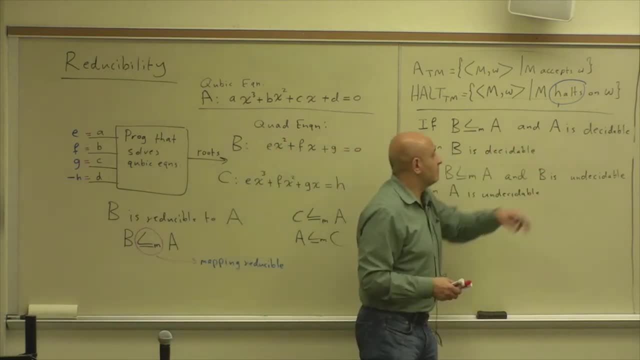 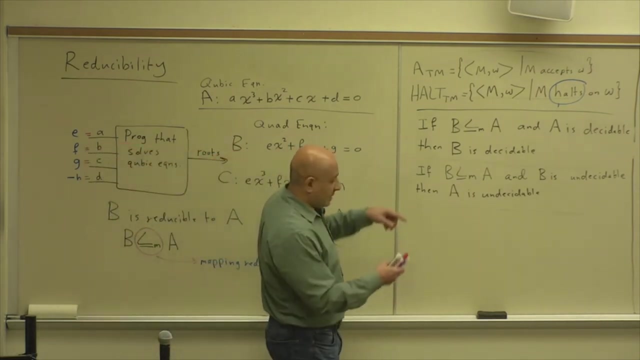 First of all, it's the contrapositive of this right. So if B is reducible to A and A is decidable, then B is decidable. This is the contrapositive. So this is the logical contrapositive. 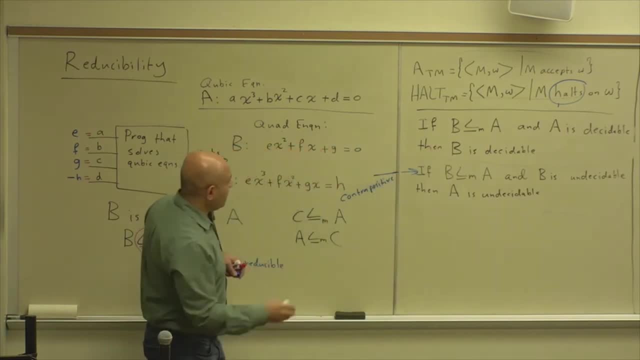 Of that. If B is undecidable, then A is undecidable. Another way of thinking of it is by contradiction right. Assume that here B is reducible to A. Now assume that we know that B is undecidable. 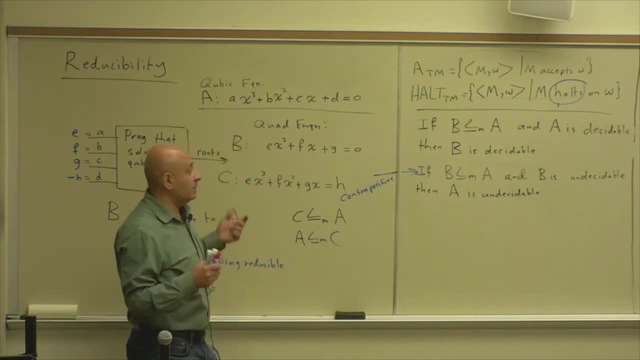 Now, if I assume that A is decidable, I will reach a contradiction, Because if A is decidable, B would be decidable, But it's not. I'm given that it's not, And the most intuitive way of thinking of this is that 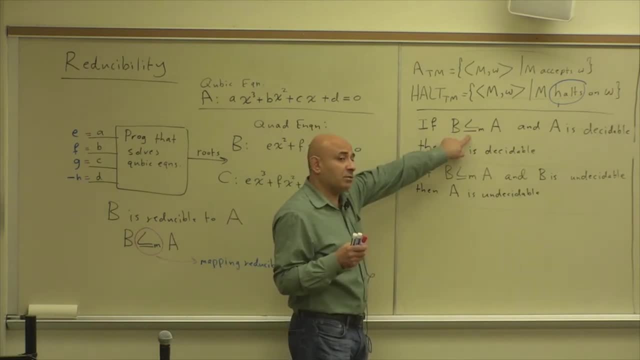 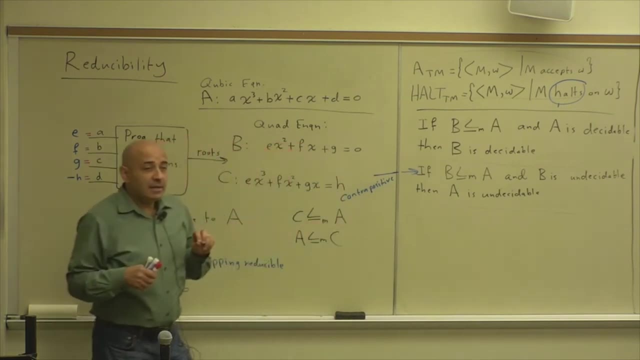 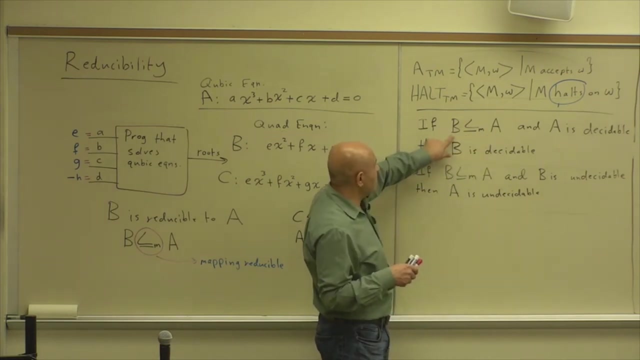 you know this mapping, this notation that we use to denote mapping. it's very mnemonic because it means that when B is reducible to A, it means that B is less than or equal to A in terms of difficulty. Okay, So B is either easier than A or at least or as difficult. 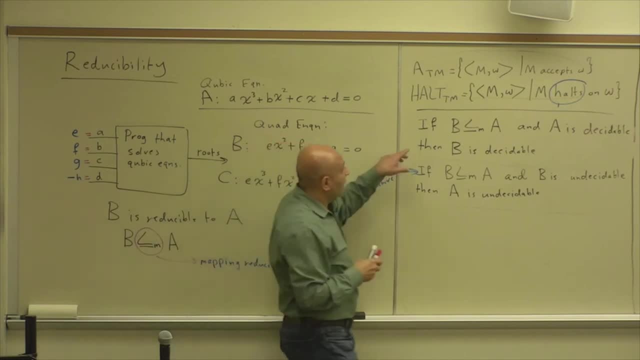 as A in terms of the difficulty of solving it. So now, if I know that the easy one is undecidable, the harder one, which is A, or the one that's at least as hard, so here, A is at least as hard as B. 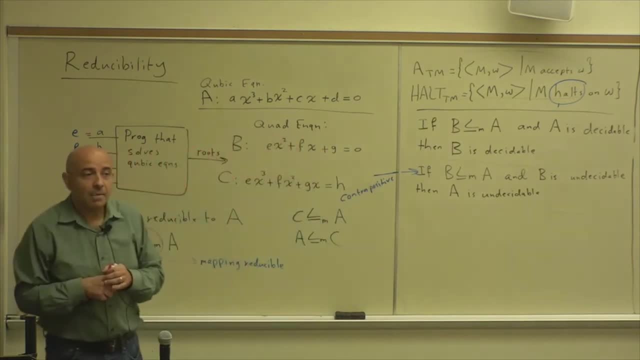 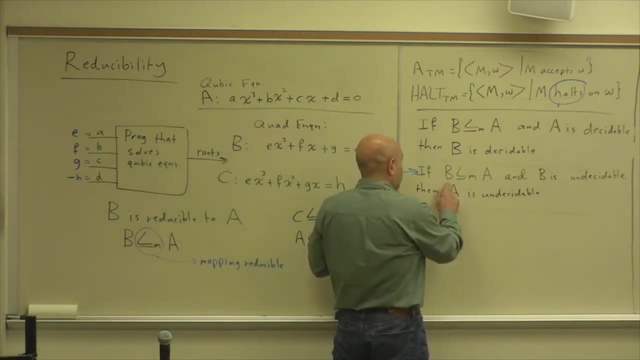 A is less than or equal to B. we can now say that A is less than or equal to B, So that the most intuitive way of thinking of this is that this problem is less than or equal to this problem in terms of difficulty. 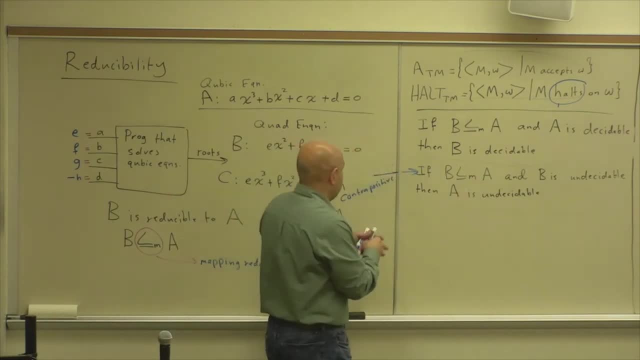 And I know that this one that can be easier or as difficult as A is not decidable, then this one must be undecidable as well. A is at least as hard as B. Okay, Now we are ready to use this to prove that the halt 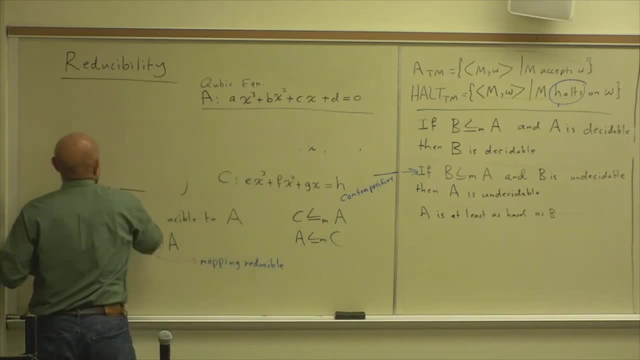 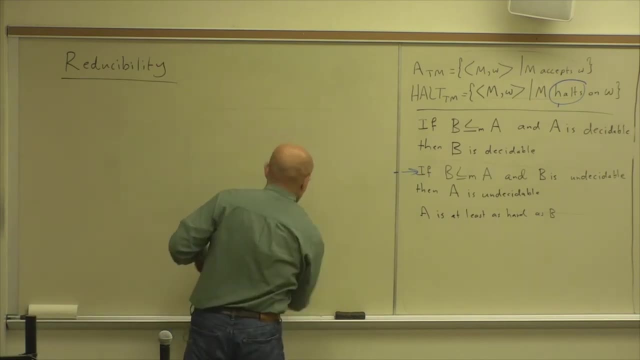 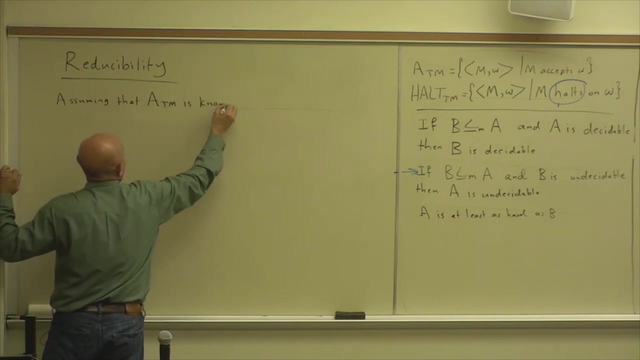 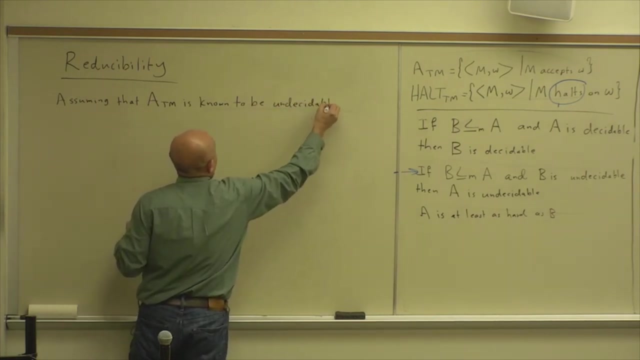 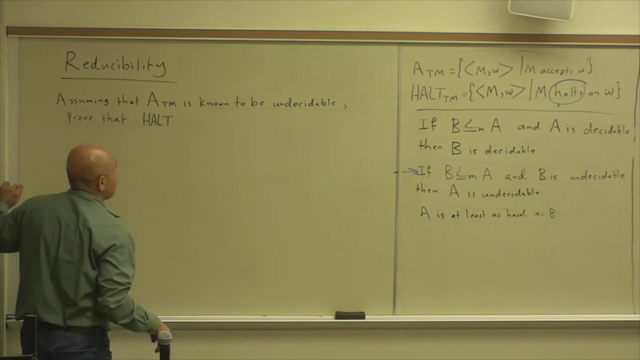 the halting problem is now. our objective is, assuming that ATM is known to be undecidable. prove that a halting problem is known to be undecidable. Halt tm is undecidable. So here you know, using the reductions, 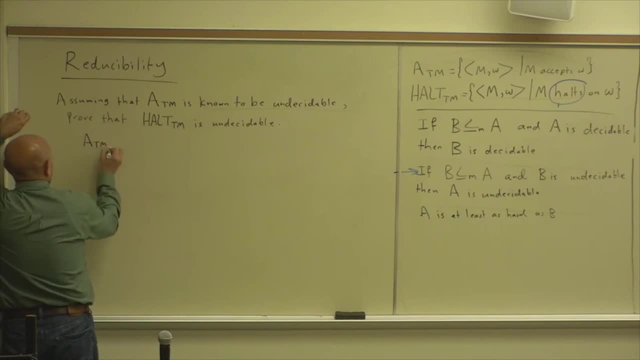 do we need a reduction from ATM to halt tm or a reduction from halt Halt tm into ATM? Which one do we need? Do we need this, the first reduction, or the second? Do we need to reduce every instance of ATM into an instance? 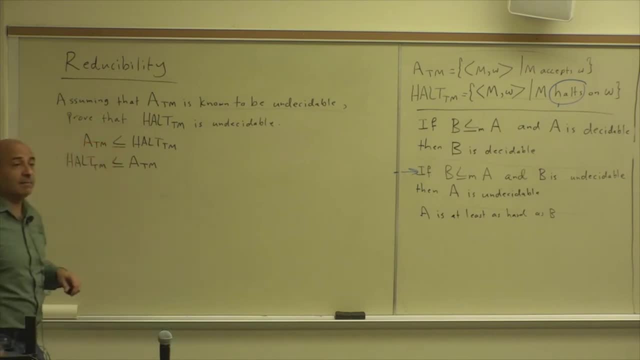 of halt, or every instance of halt into an instance of ATM. Why is it the first one? Because if the one at the beginning is less than or equal to 8.. Yeah, this is the one that will help us show that halt tm is undecidable. 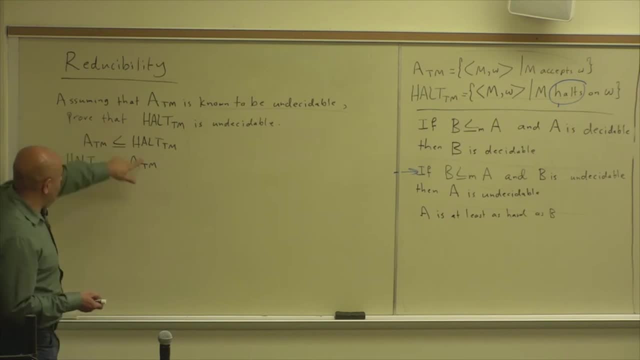 If the if ATM is less than or equal to halt tm in terms of difficulty, or halt tm is at least as hard as ATM in terms of difficulty. this will help us prove that halt is also undecidable Because a problem that's less than or equal to it. 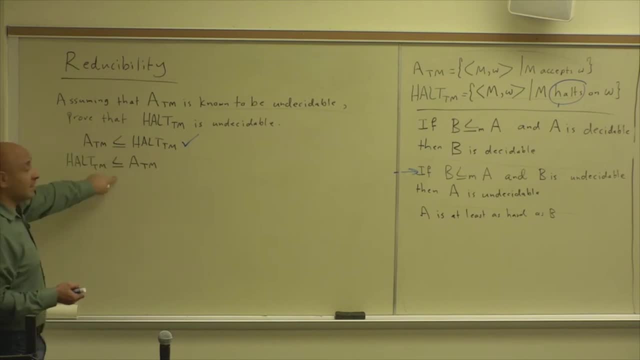 in difficulty is known to be undecidable, While if we show this, it will not prove anything. Right, This will not prove anything. It's like you know, this is known to be hard, And if we show that, halt tm is less than or equal to a problem, 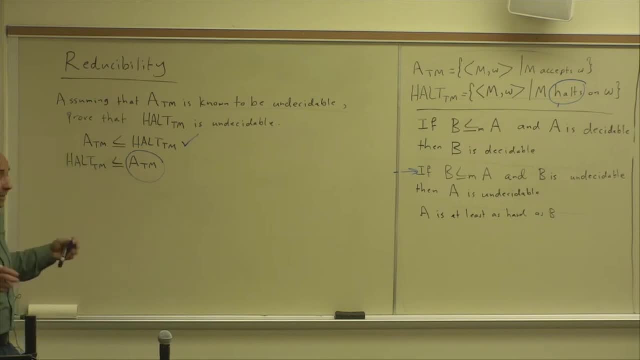 that is known to be hard. less than or equal to it in terms of difficulty, that will not prove anything, Because this can be much, much easier, Right. So showing that it's less than or equal will not help us prove anything. 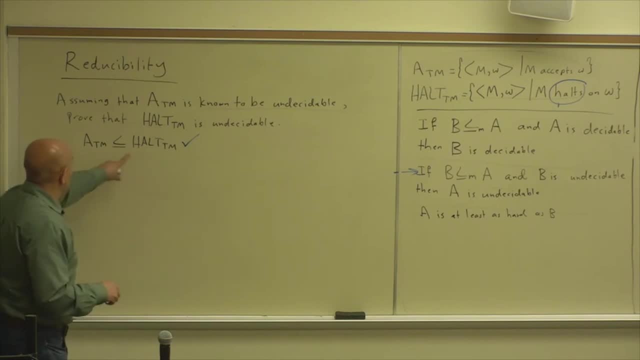 Okay. So now we need need a reduction from ATM to halt tm. So we need to show that need to show that we can reduce every- or sorry, not reduce- convert. We can reduce every instance of ATM into an instance of halt tm. 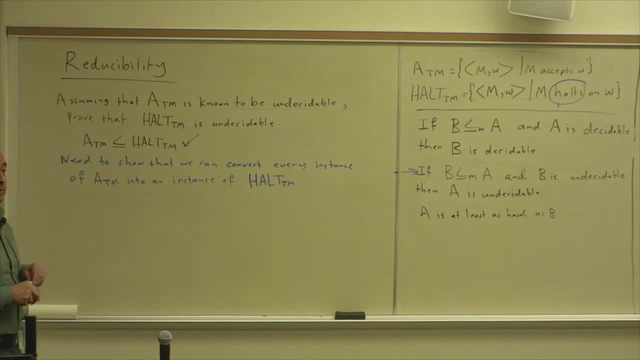 How Well, let's think about it in terms of programs first, before we think of it in terms of Turing machines. Now, to convert every instance of ATM into an instance of halt tm, I will have to assume that I have a solver for halt tm. 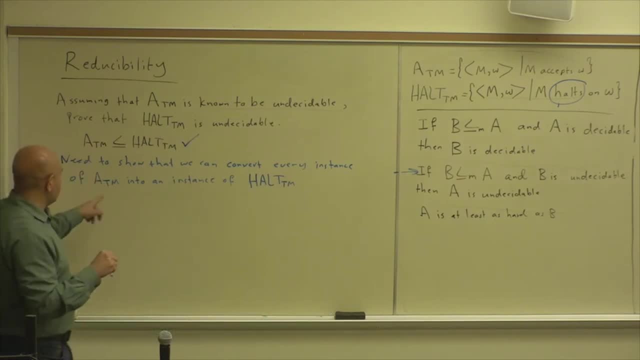 So, assuming that I have a solver for halt tm, I can use it to solve ATM. So I'm going to show that if I assume that I have a solver for this, I can solve any instance of this, And then this will contradict. 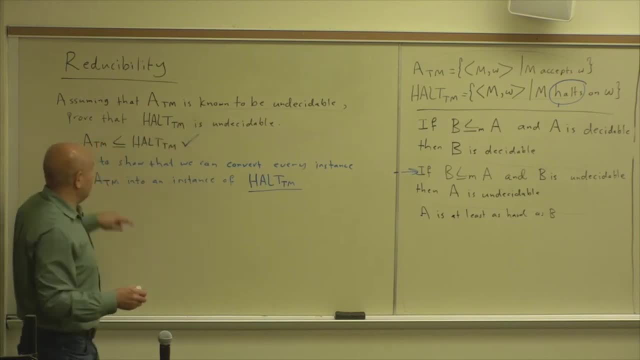 What is the solution? What is the solution? The solution is given, which is ATM, is not solvable. So you assume that you have a Turing machine R that decides a halt tm. So let's think of it in terms of programs. 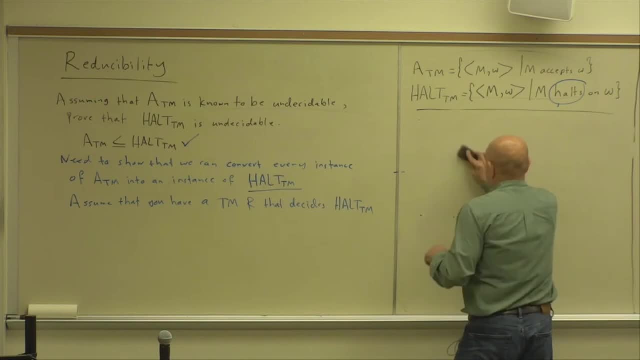 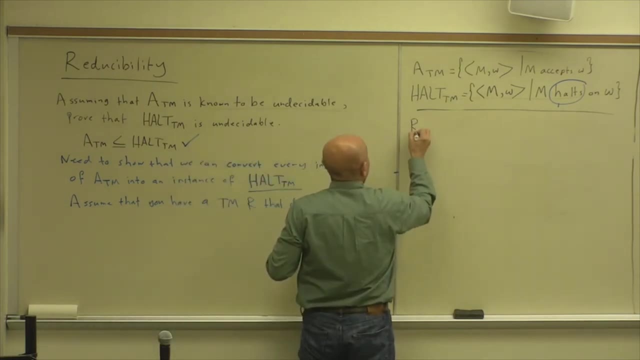 So R, just a program, R that takes another program, M and W, And it tells you if you know, if M holds somehow with some magic. If M holds M somehow with some magic, algorithm halts on W return, yes, else return, no. Now I'm assuming that I have this magical. 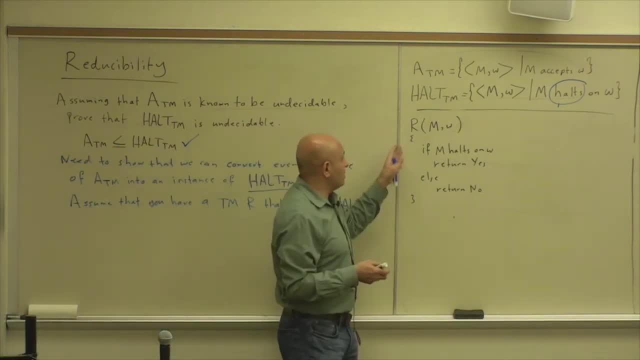 program or this magical algorithm that solves the halting problem. I give it any program and any string and it tells me magically. Of course we will reach the conclusion is that such a program cannot exist. But now we are assuming that it exists, and then we 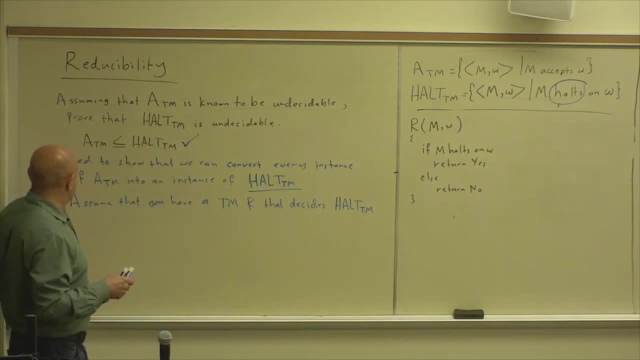 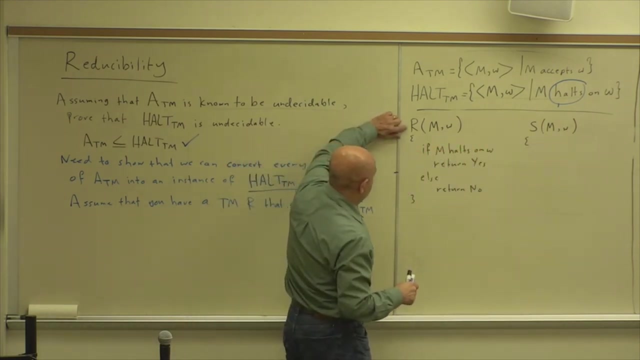 will reach a contradiction with what's given, which is ATM is not decidable. Now let's assume that we have this S that takes M and W and we need to use this to determine if M accepts W. If you use this solver for the halting problem to solve the acceptance problem, all what? 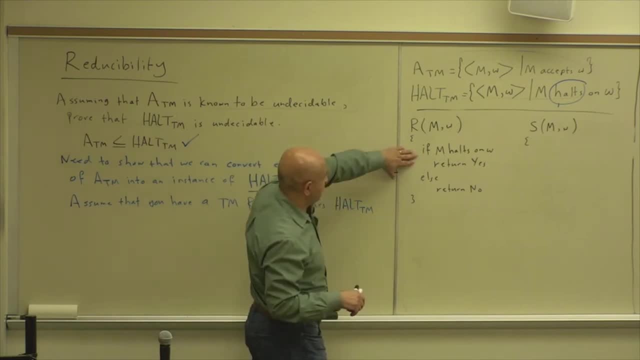 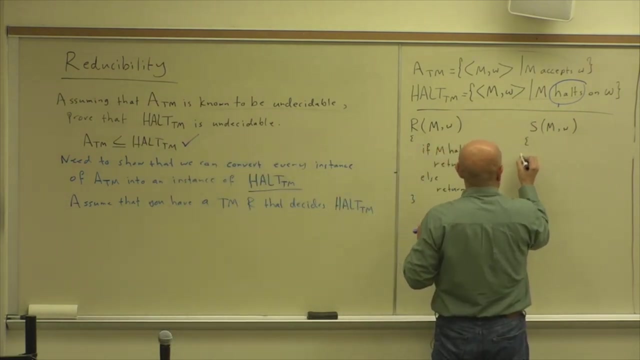 you need to do is to call this to determine if this halts or not. If it halts, then you call the, then you run M, If it doesn't halt, you just reject. So what you need to do here- sorry, I was thinking in another problem- So if you know, run R. 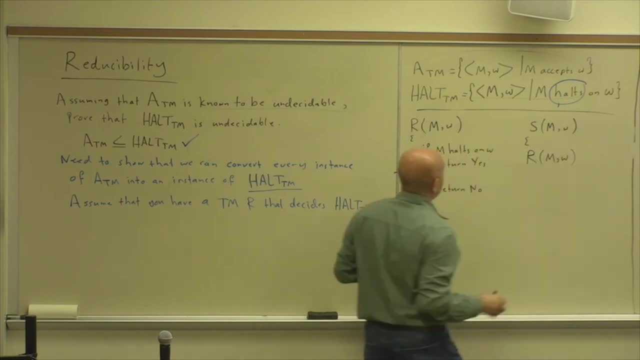 Of M and W. you run R Or if, and this is the result of R. If. result equals no, reject, Else what No? No, No, No. Now if R rejects. if R says no, it doesn't halt, then I reject the string. Now if it. 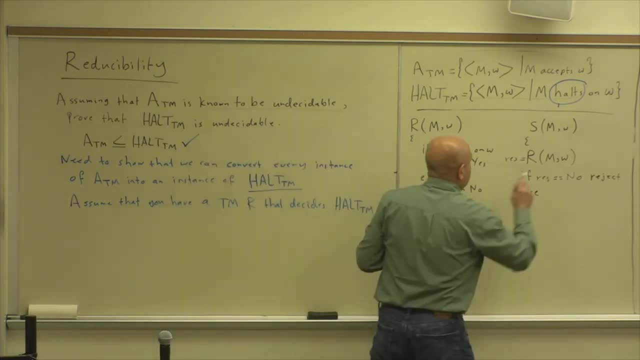 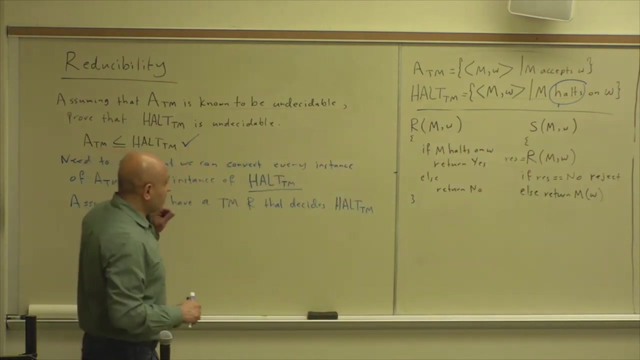 doesn't reject, if R does not reject or if the result is yes, it means that it halts and it will be safe to call M Else, just run, just call or return M of W. So, assuming that this magic program that determines if a program halts or not exists, it can help. 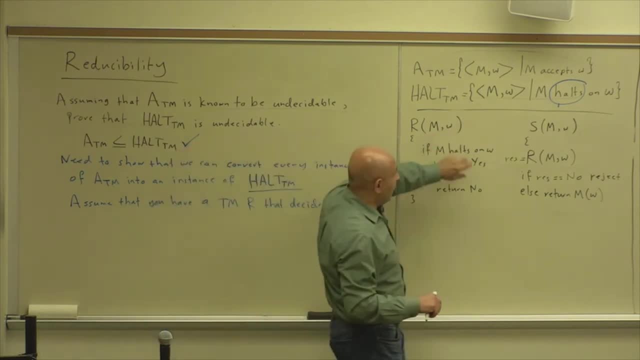 me avoid looping forever Because I can call R and it tells me if R is going to loop on the string. If it tells me with some magic that it's going to loop on the string, then I'm going to reject it without having to loop forever. Otherwise, I will just call M and 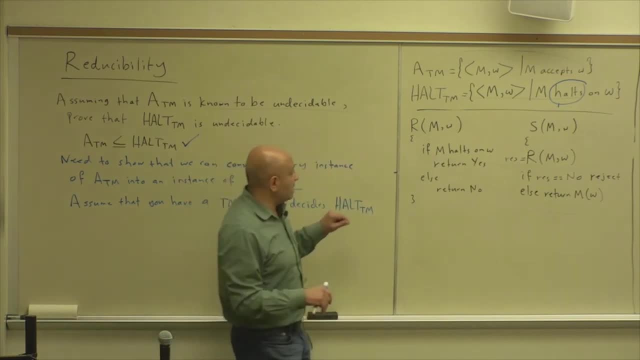 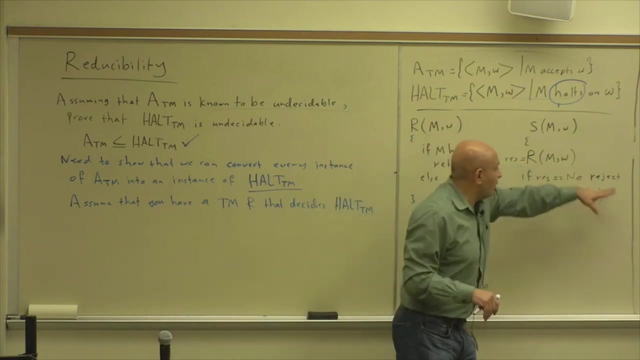 I know that M in this case will terminate. Why? Because this magical R told me that M halts on W. So in the else part I'm guaranteed that M is not going to loop, Because if it loops I will reject. Otherwise I will return. 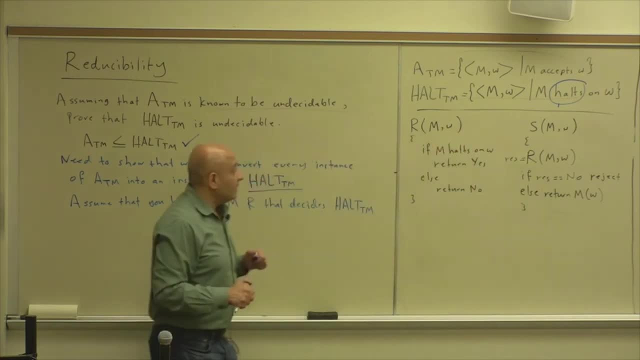 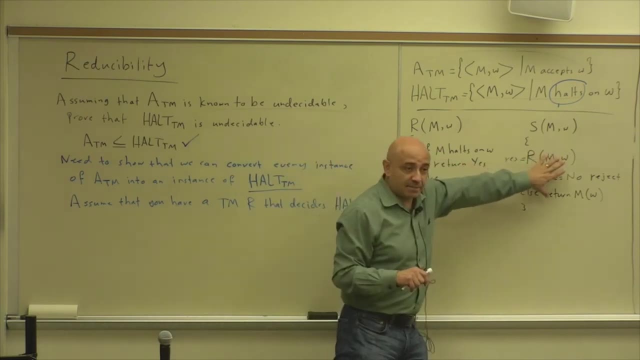 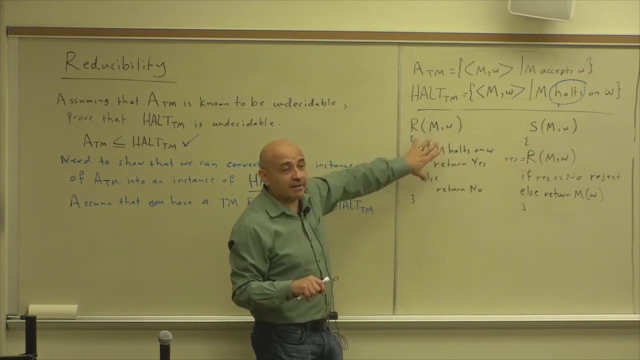 M. So this is. this means that if you give me a solver for the halting problem, I can use it to solve the acceptance problem, But I know that the acceptance problem is undecidable. Therefore such a solver cannot exist. So I conclude that this solver cannot exist, Because if I have it, I will be able. 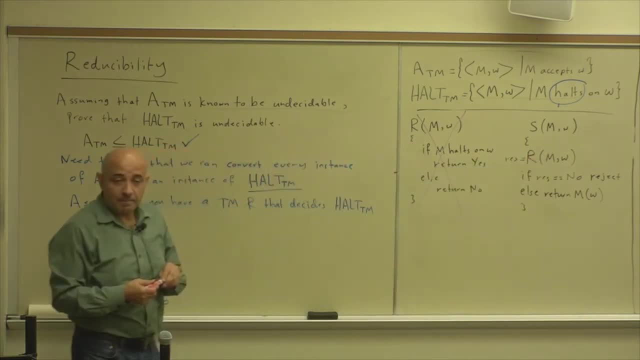 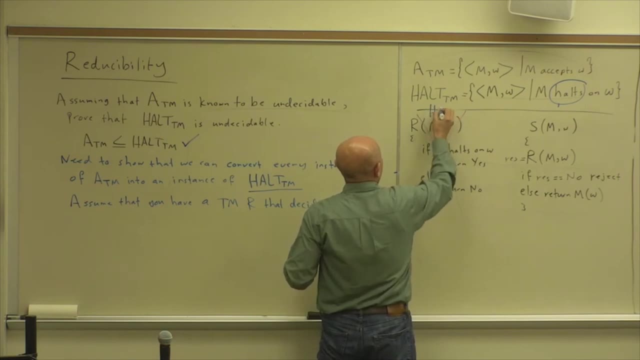 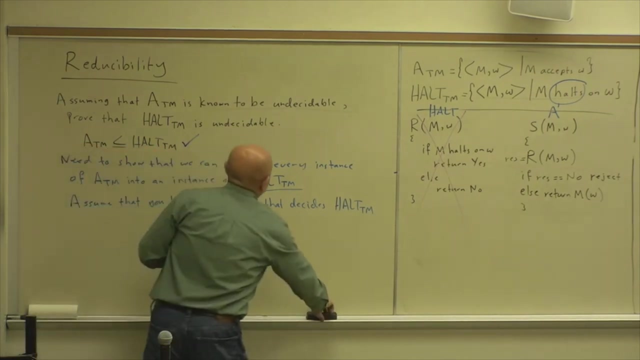 to solve ATM with it. So this is a, you know, this is a solver for halt and this is a solver for A acceptance. Okay, So we can write this in terms of a Turing machine. now, You know, given, okay, assume. 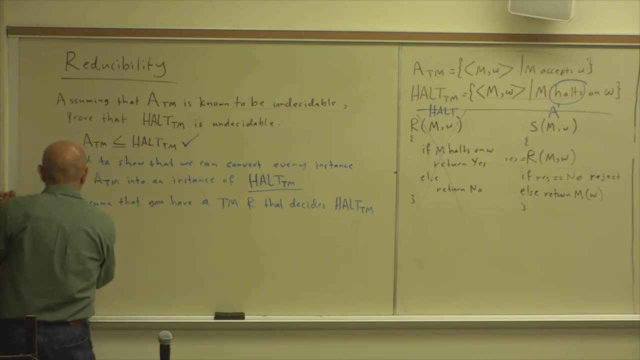 that you have a Turing machine R that decides halt. We can build a Turing machine S that solves ATM as follows: Okay, Okay, Okay, S is going to be run R on W, Run R on M and W If R rejects or if R says that it doesn't. 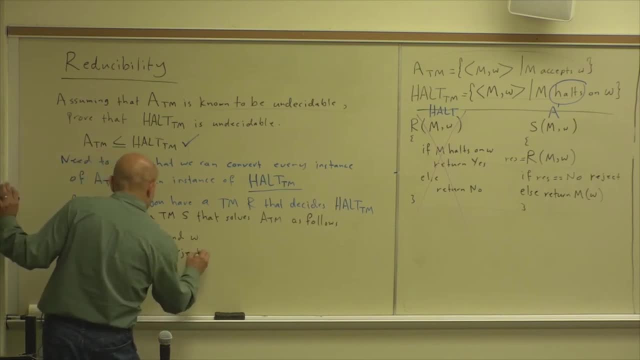 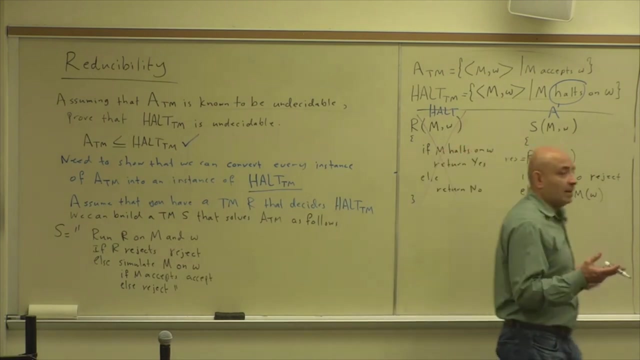 halt, rejects, reject, else simulate M on W. If M, M accepts, accept, else reject. So basically, you know, this kind of conversion or reduction is very similar to the reduction of the two different forms of cubic equations, because these two problems are just very similar. 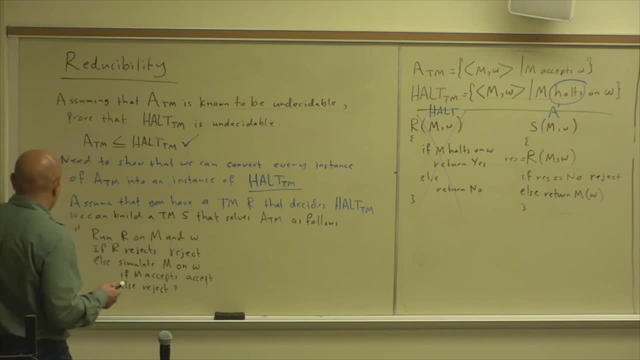 So here what we are saying is: if we have a solver for HALT, we can build a solver for acceptance ATM, But we know that such a solver does not exist because this is undecidable. Therefore, a solver for HALT cannot exist. 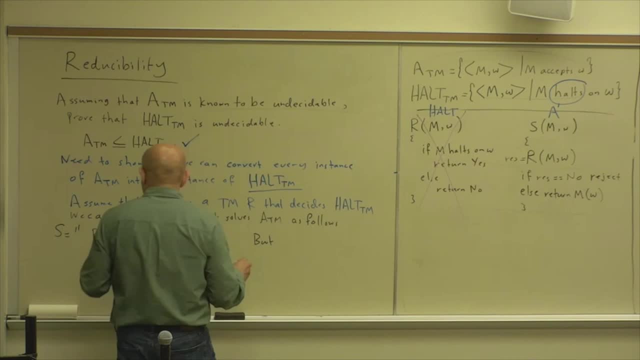 But this contradicts the assumption that no Turing machine That decides ATM exists. Therefore, you know a decider or decider, R for HALT. you know R for M for HALT. you need for HALT. Sorry to-to guide. 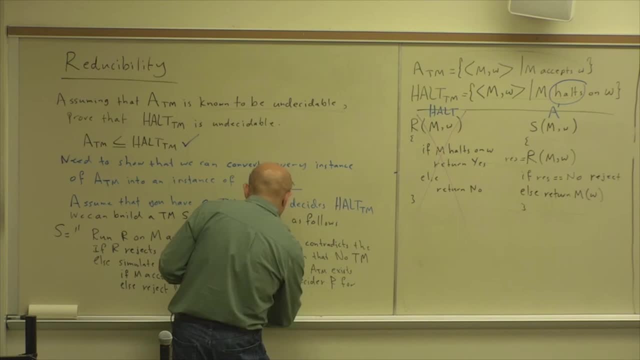 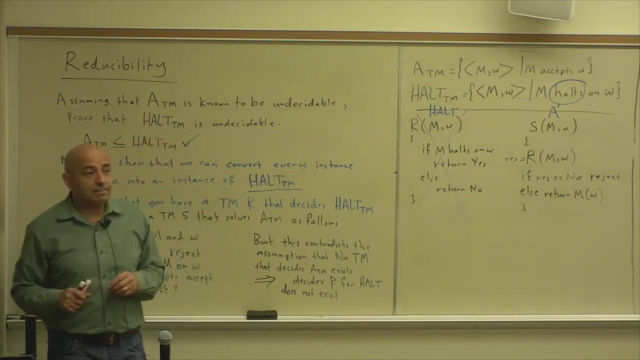 Yes, thous Yes for HALT. decider R for HALT does not exist. Okay, So basically we're showing that you know, HALT is not any easier than ATM, And if you give me a solver for HALT, I can use it to solve ATM. 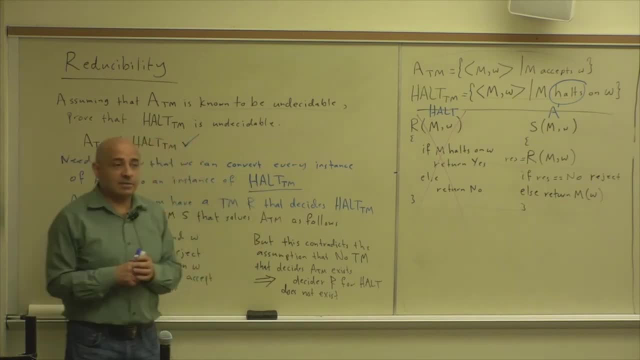 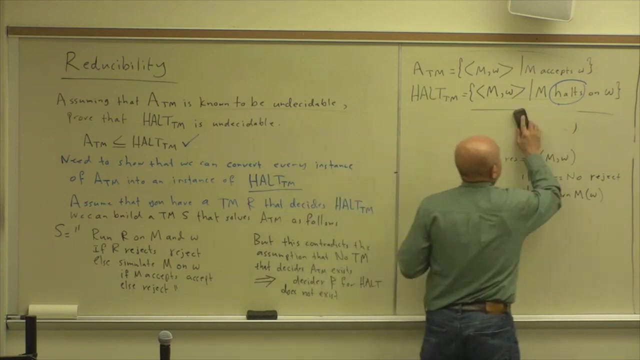 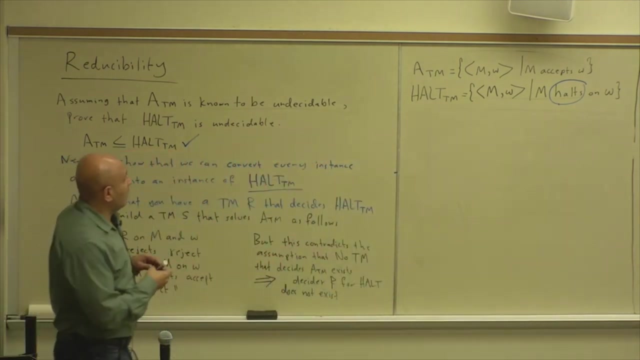 But since ATM is known to be undecidable, the solver for HALT cannot exist. Okay, So now any questions on this. Okay, So on this topic, you know, things take longer than expected. Okay, So now we will look at the emptiness problem, MTTM. 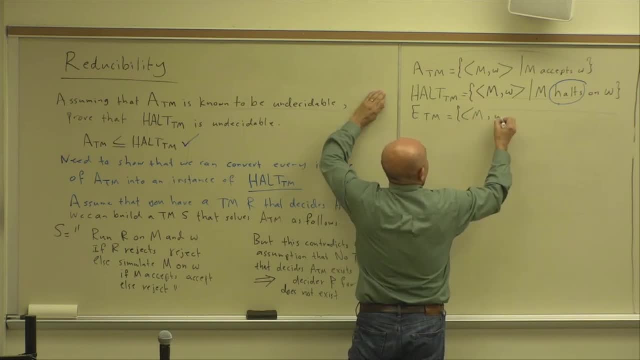 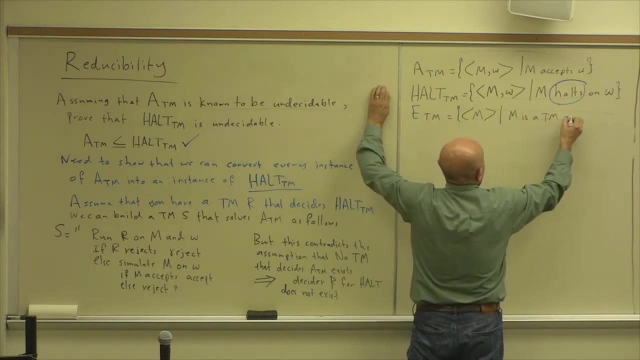 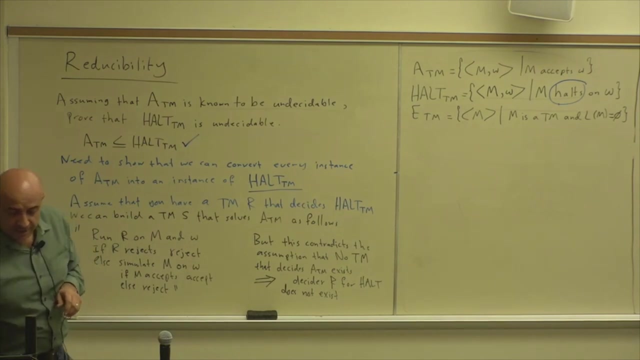 where we are given M and only M, And M is a Turing machine and the language of M equals phi. So this is a problem that we managed to solve for finite automata and regular languages. Is it solvable for Turing machines? The answer is no, because we can reduce ETM to 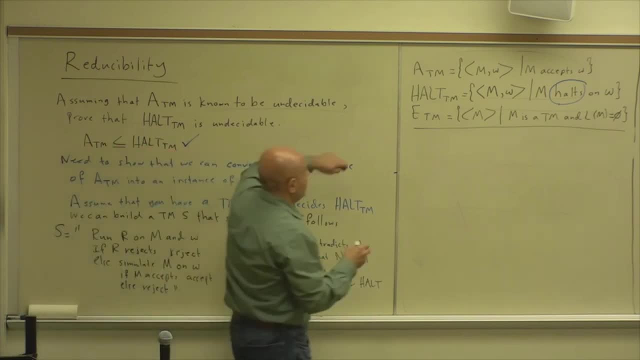 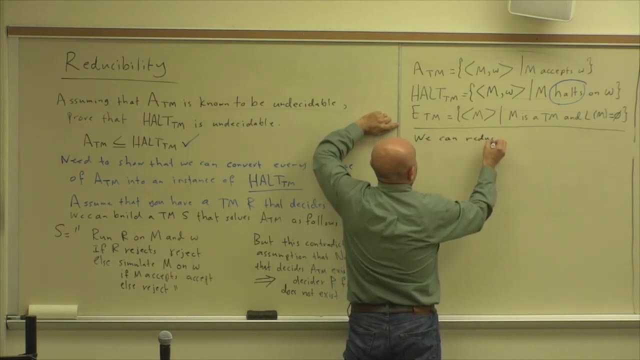 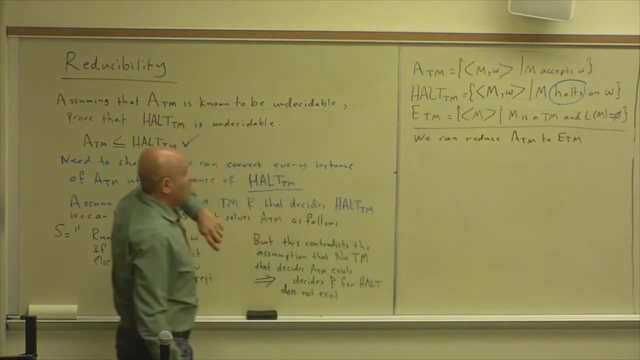 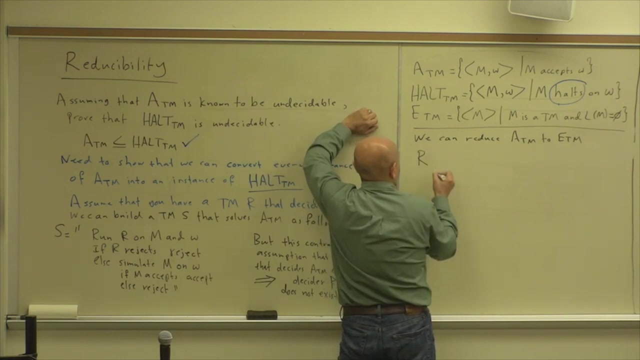 or we can reduce ATM to ETM, So we can reduce ATM to ETM. Or if we are given a solver for E, we can solve A. So this solver R for ETM, it takes a machine R and it returns. you know, it returns yes. 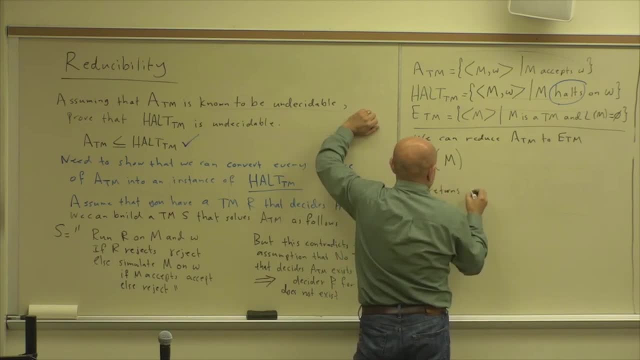 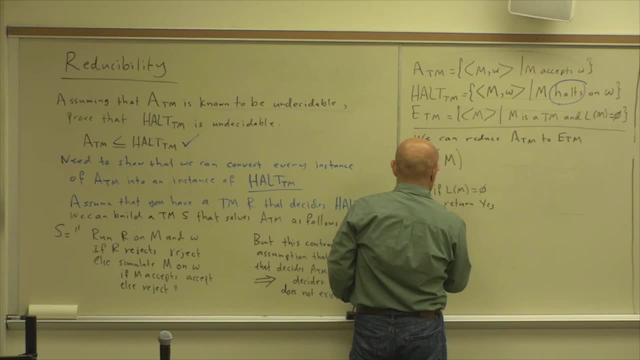 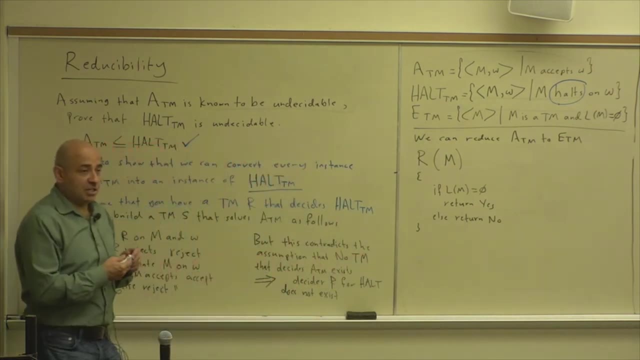 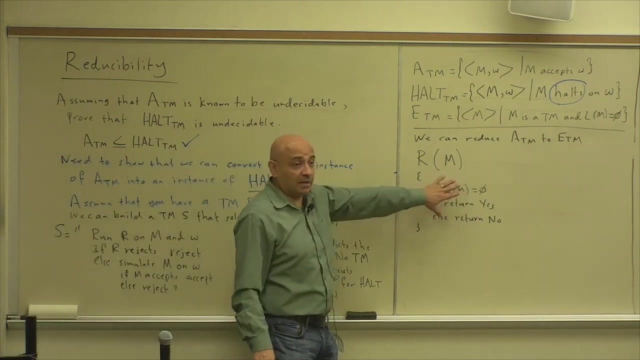 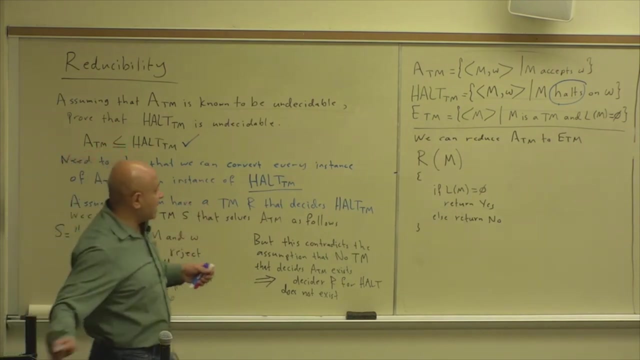 Yes, Yes, Yes. Now again, this is a magical machine that we assume to exist, but then we will conclude that it doesn't exist, Because if such a machine existed, we can use it to solve ATM. So how can we use this to solve ATM? the acceptance S. 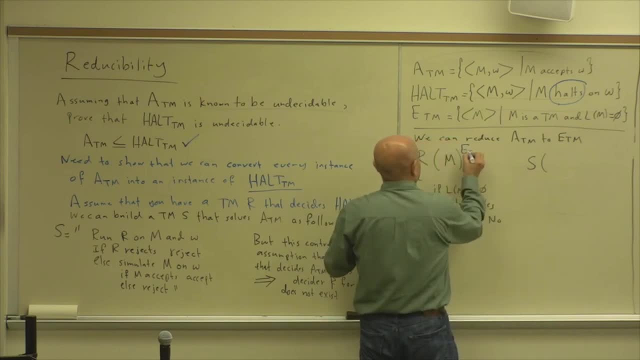 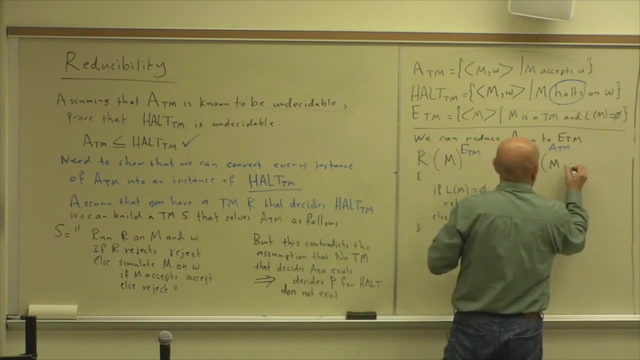 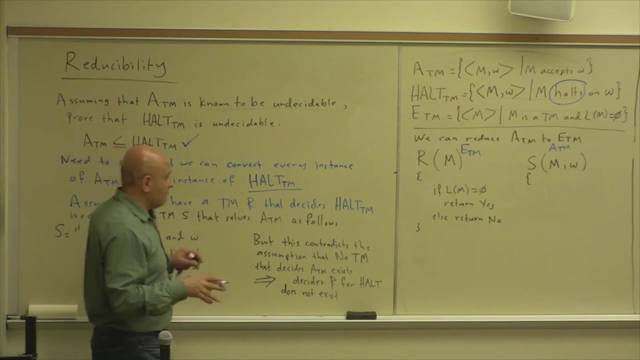 So this is ETM and this is ATM. So this takes M and W. Now this is where we need to construct, you know, to transform M into another machine, Because if this tells us that, you know, if we call R and it tells us that, it says: 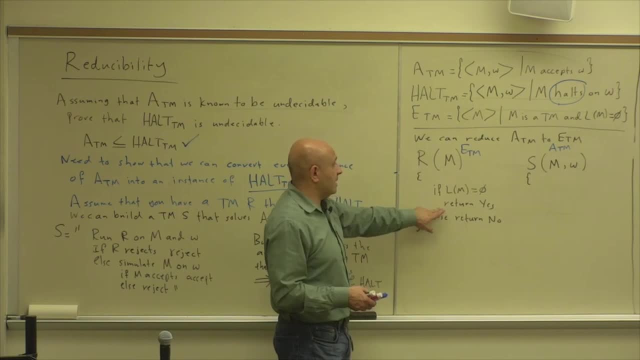 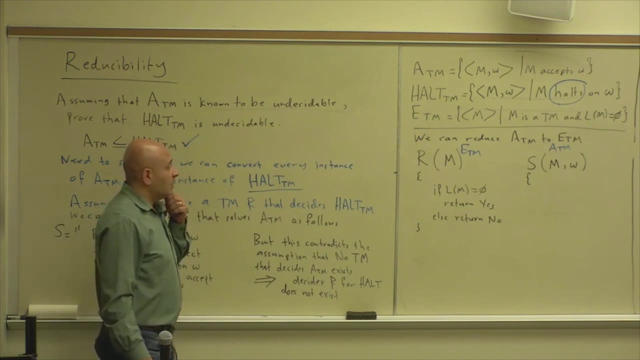 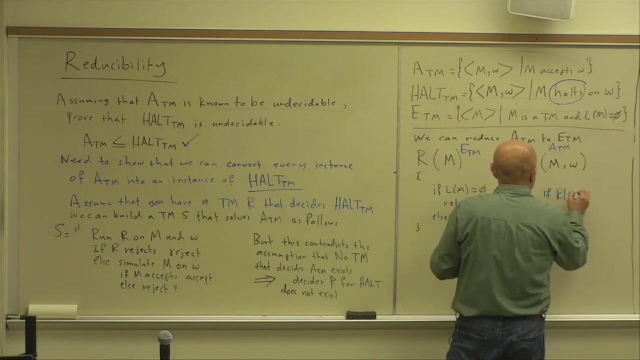 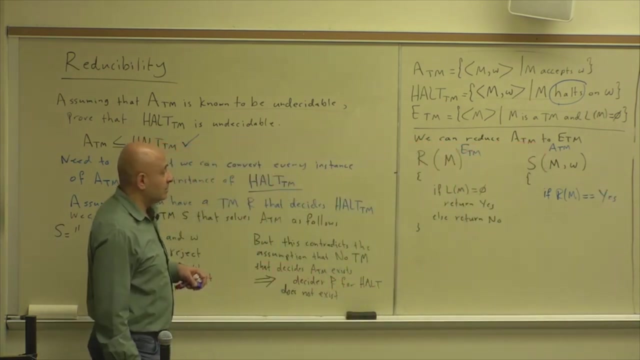 okay, Yes, if we call R and R says yes, what should we do? What should we return for W? So we're given M and W and we call R of M. If R of M equals yes, what should we do? 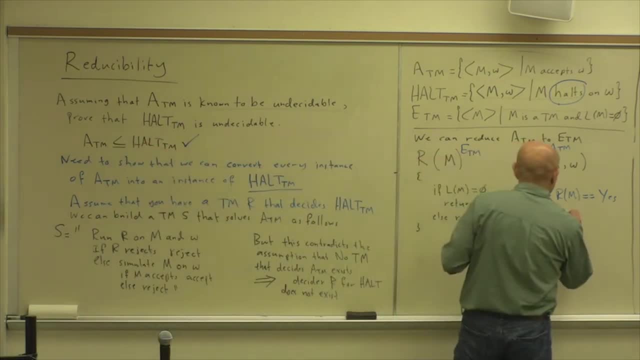 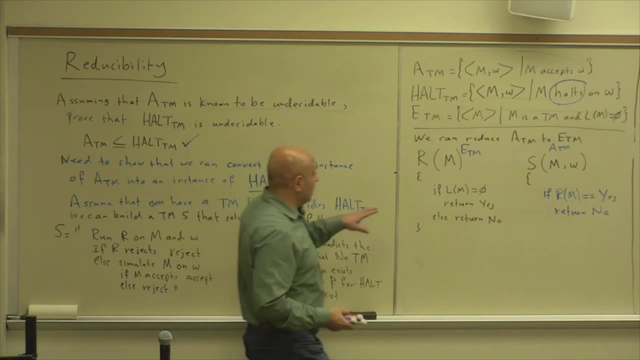 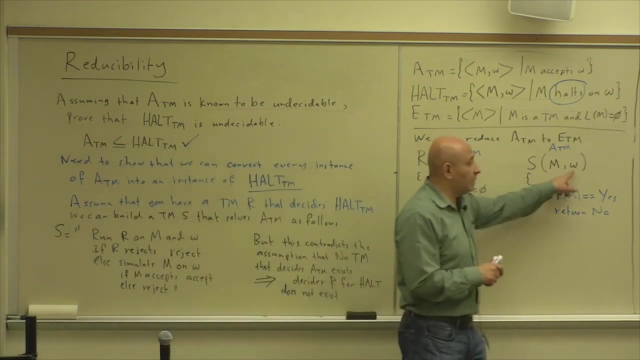 Return no, definitely. If R of M equals yes, we return no, Because this means that M does not accept anything right? So if this magical machine tells us that this M rejects everything, then it will reject W, But if it tells us no, does this help us determine if M accepts or rejects W? 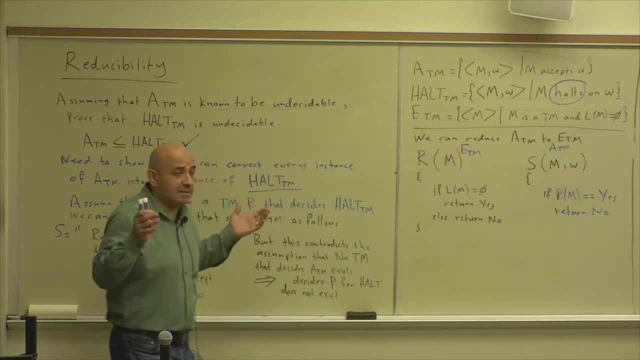 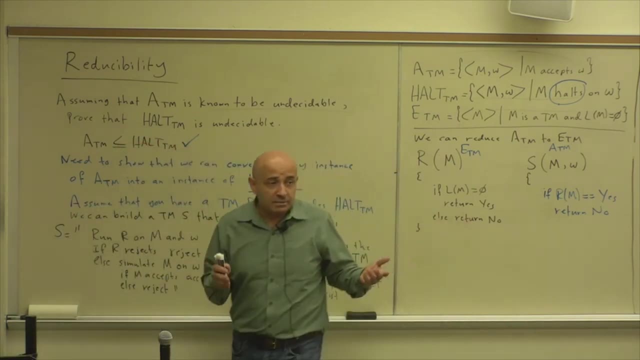 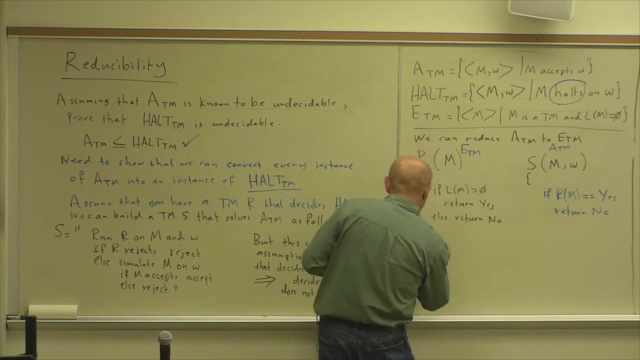 No, it will not. It says it just accepts some strings, Okay, And W can be one of those, sub one of those strings that M accepts but and it cannot. Now, this is where we need to transform M into another machine, M1, that takes X and it. 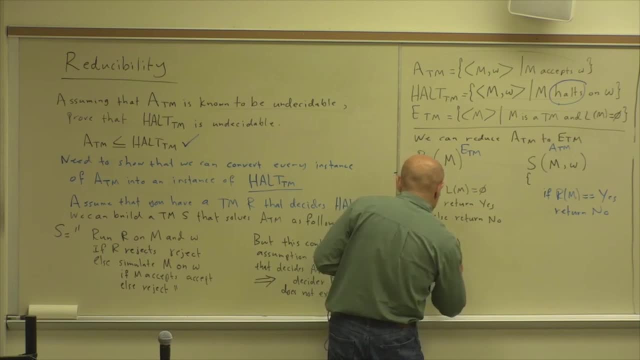 says: if X equals W, X does not equal W return. no, It says: if X equals W, X does not equal W. So it says: if X equals W, Y does not equal W, X does not equal W. and it says we need. 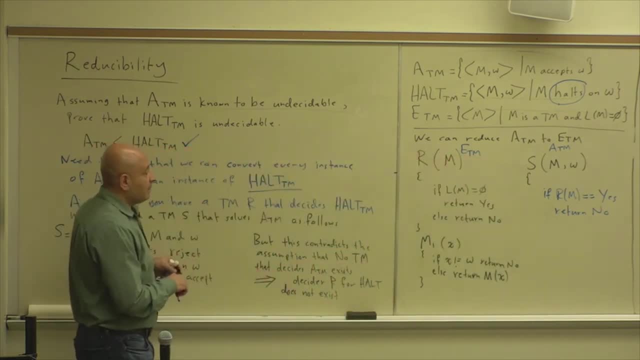 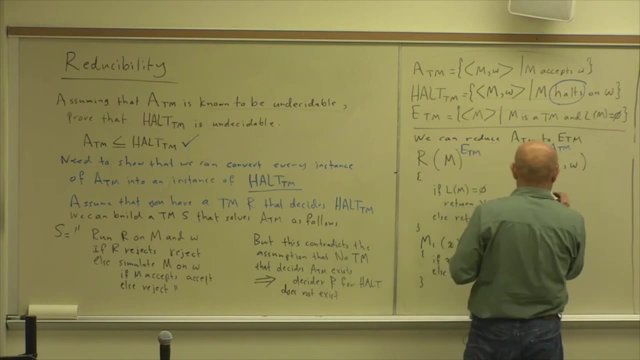 to return M and W. Now if we say if X equals W, then all right. so after we return M and W, we'll return the M here, because at the end of the function we're going to return M And where we're going to return M. 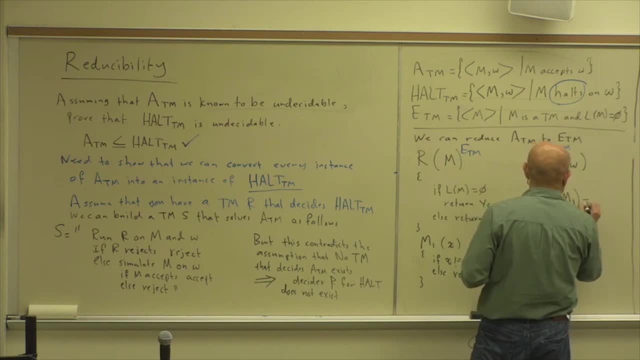 J, Yes, Or return, sorry, M of X. Now, if I call R, well, first, if called, if R of M equals yes, I want to Здесь return M and I'm going to return m of M1 equals no. 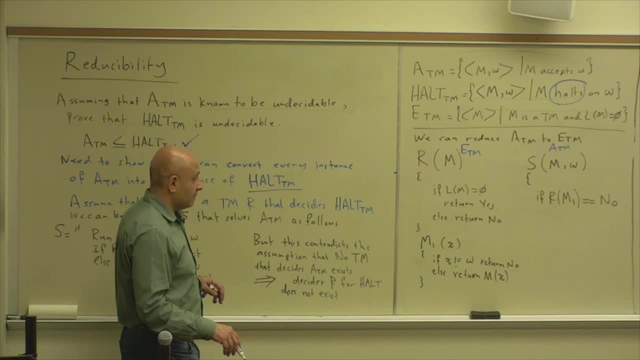 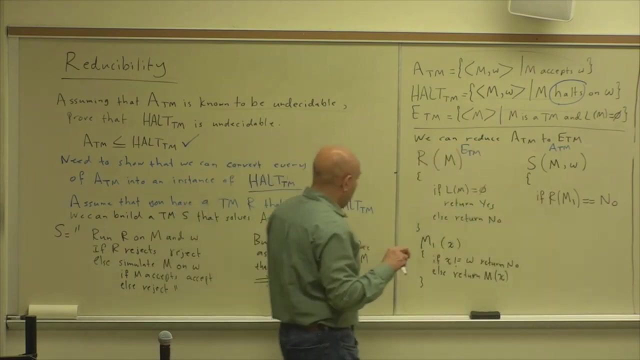 What does this tell me? If R of M1 equals no, Okay, Now does this help me solve this? Now, what if R of M1 says yes? Then I know for sure. if R of M1 says yes, I know that M accepts W, Because M1 cannot return yes unless the